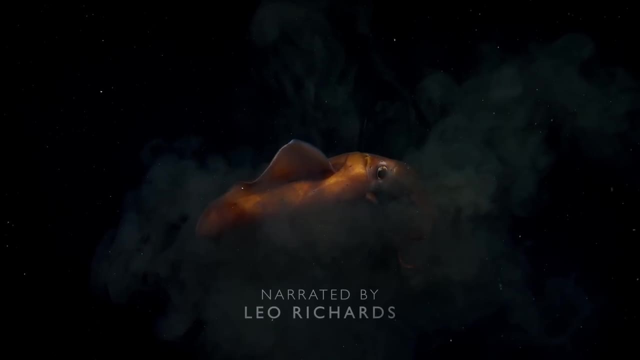 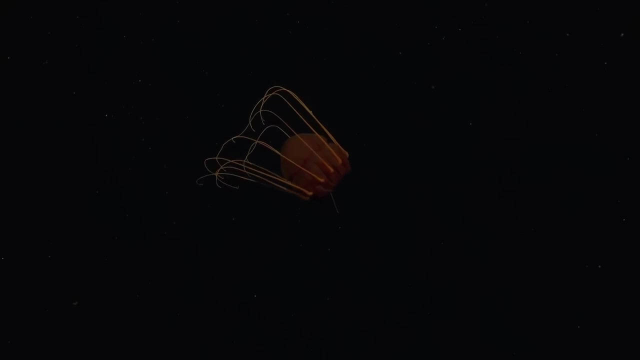 With every new discovery that is made in this fascinating world, we come a little closer to understanding the processes at play and the more complex it starts to appear. In 1843, naturalist Edward Forbes proposed the Abyssus Theory, in which he 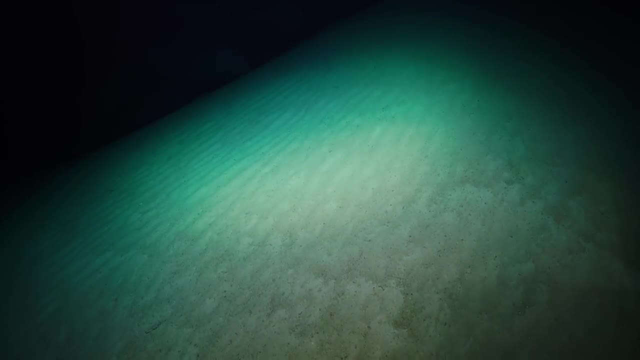 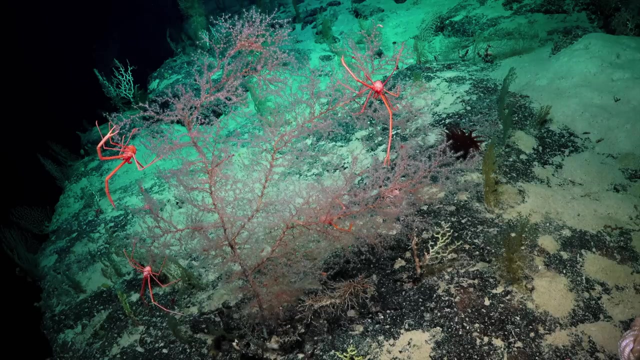 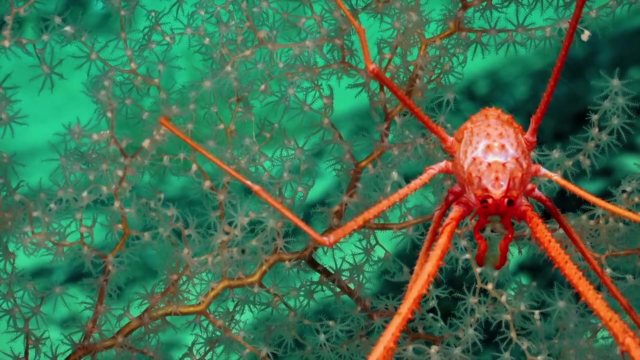 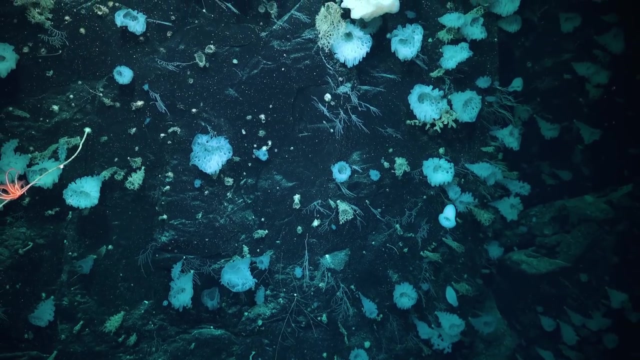 postulated that the abundance and variety of marine life decreases with depth and altogether ceases. Of course, this theory is long superseded and we know now that the depths are home to remarkable biodiversity existing across an array of interconnected worlds. In the deep sea, life is concentrated at chemosynthetic oases. 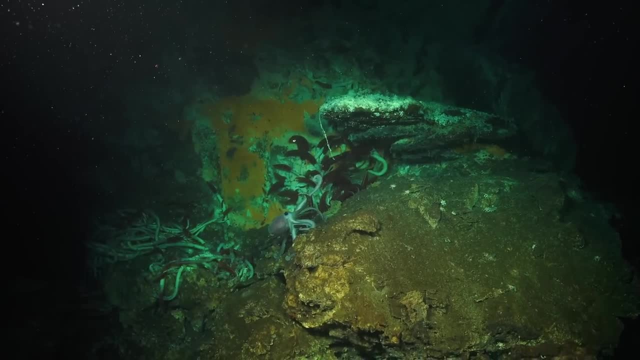 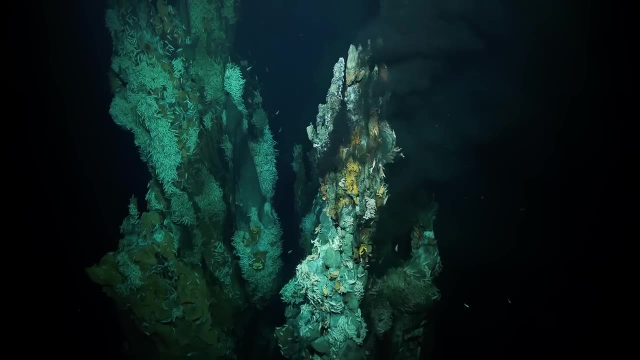 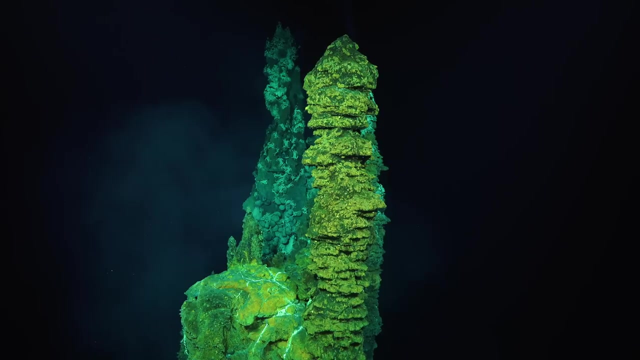 and communities that form, where primary production is made possible via chemosynthetic oases, with bacteria converting hydrocarbons into food at cold seeps and hydrothermal vents. And although these oases are hotspots for life, treasures can still be found. 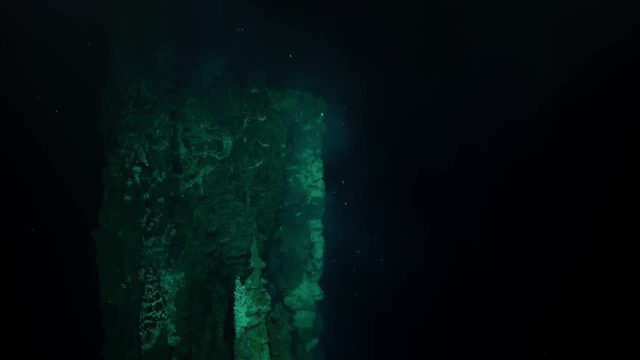 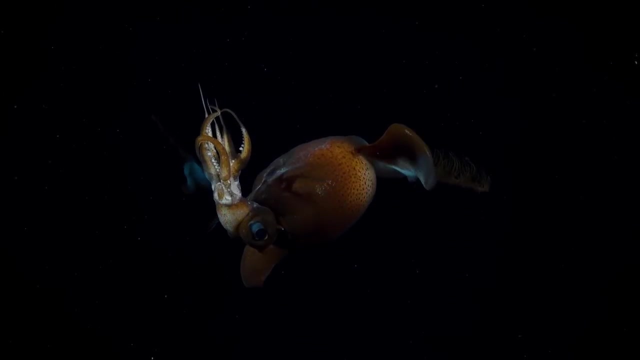 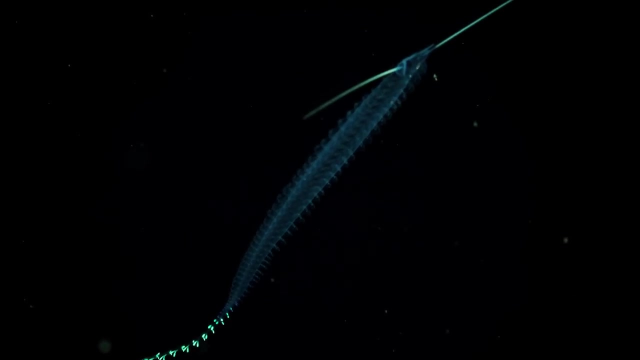 elsewhere in the deep sea, but adapted to an entirely different set of challenges. The non-chemosynthetic regions of the deep are divided, and there is no way to know which is which. They are divided into two very different worlds. First is the midwater, an ecosystem that encompasses the water column. 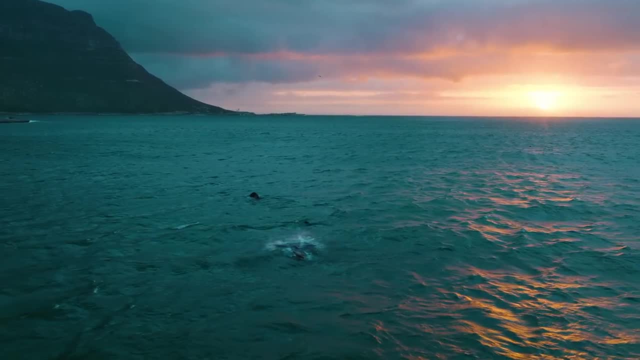 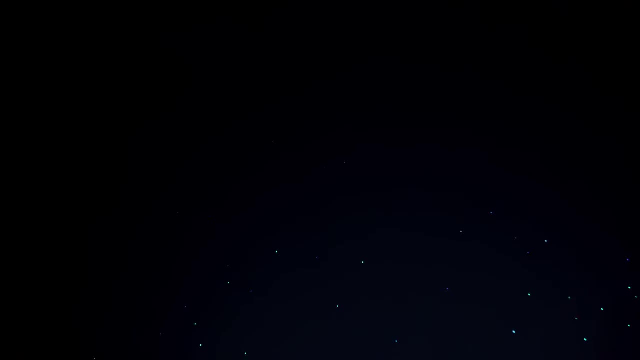 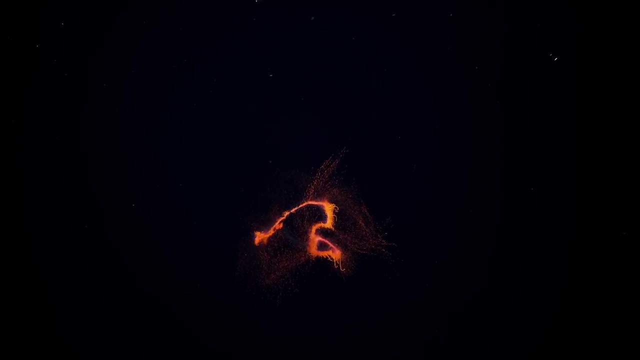 where pelagic wanderers tread migratory routes that span entire oceans And planktonic drifters and their predators take part in bioluminescent light shows glimpsing in the dark Suspended drifting, moving in tune with the current, the ocean's. 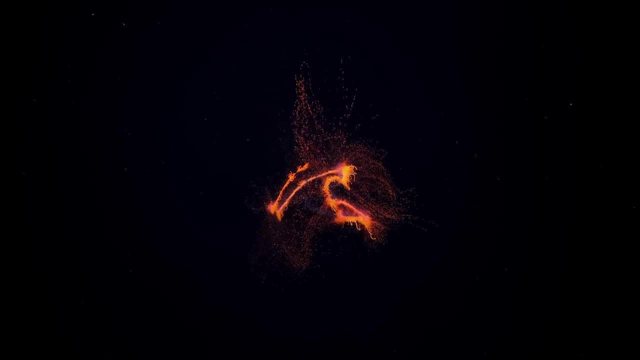 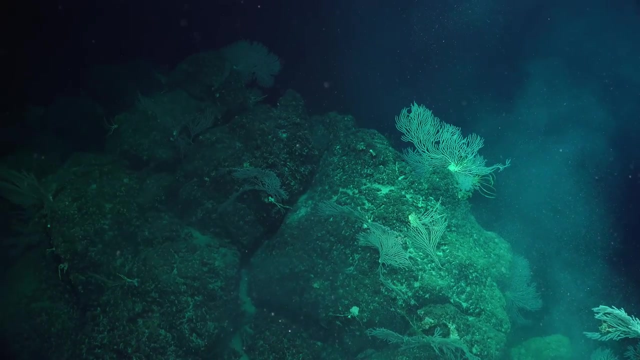 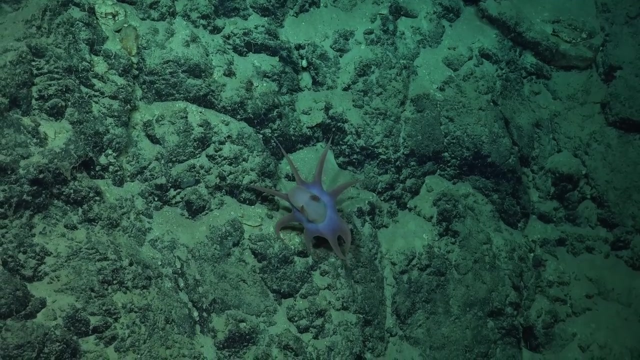 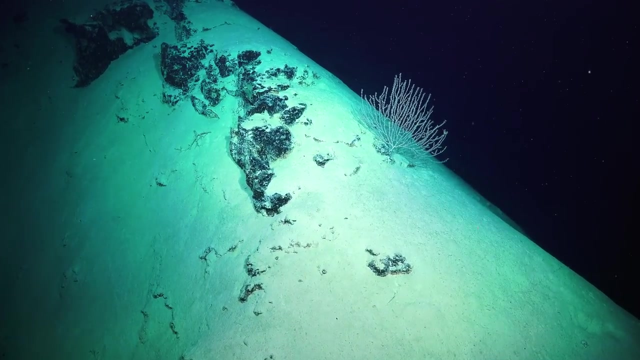 guide to the elements around it, and below lies the deep, dark benthos, The world of the deep sea. floor like the surface of an alien planet, A kingdom of mud and ooze where sessile creatures cling to any solid outcrop. 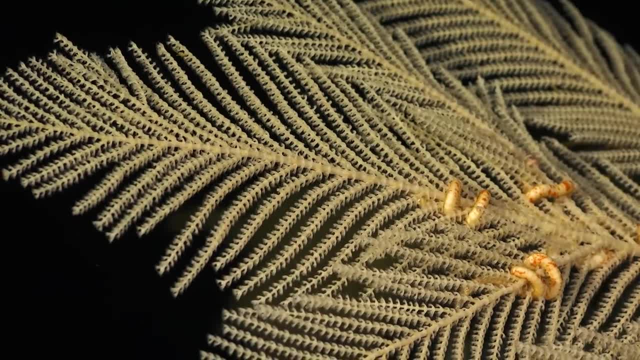 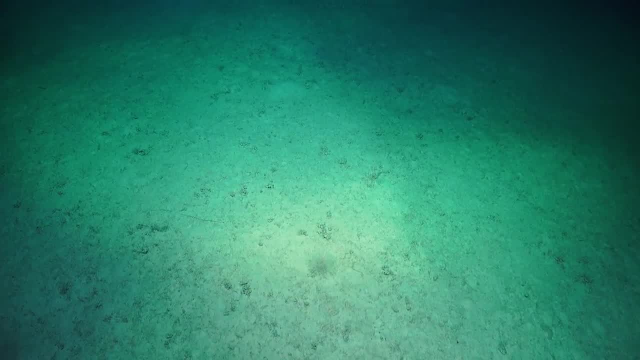 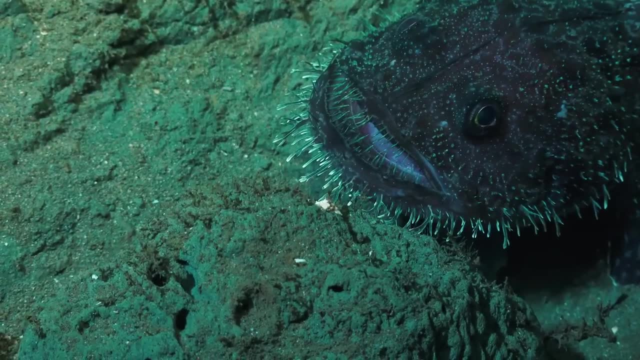 they can find, reaching hungrily into a shower of scraps and debris. The deep sea floor is at first glance a place of filth and decay, destitute perhaps and full of horrors. But if we look a little closer, we uncover a place of beauty. 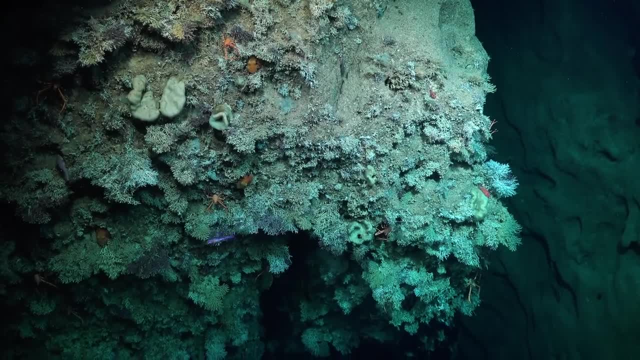 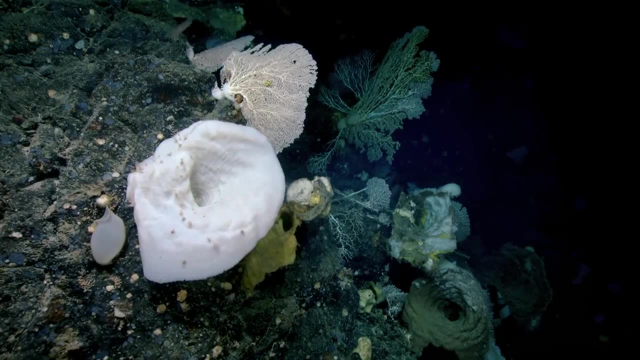 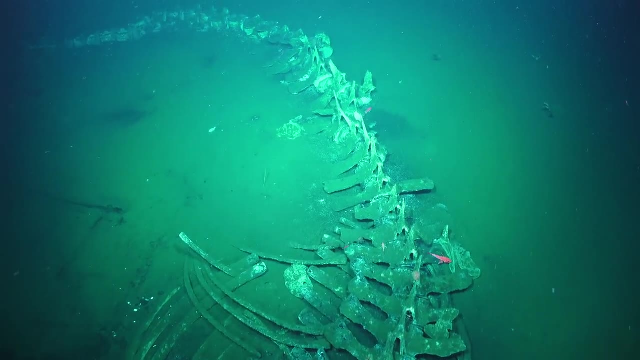 A realm where corals craft mighty kingdoms on the seamount crusts, Where the delicate structures of sponges provide refuge for others And where scavengers attend bountiful feasts that last for decades. The two worlds of the deep could not be more different. 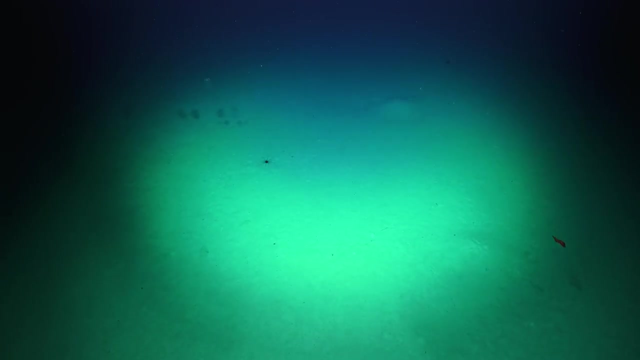 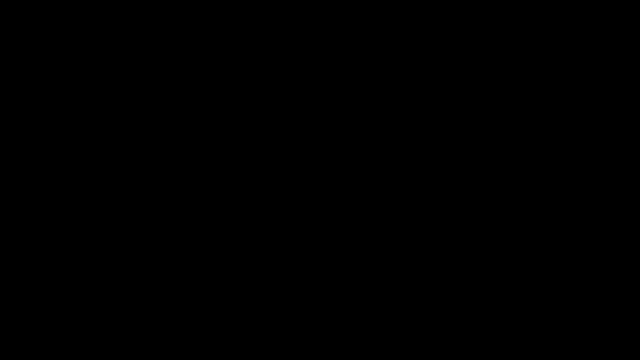 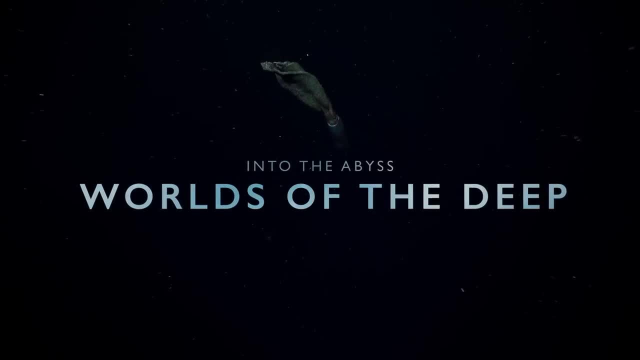 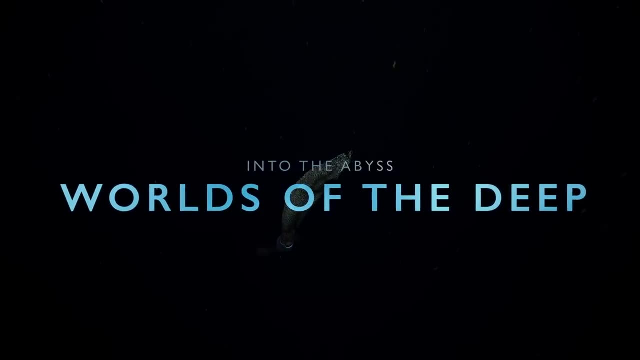 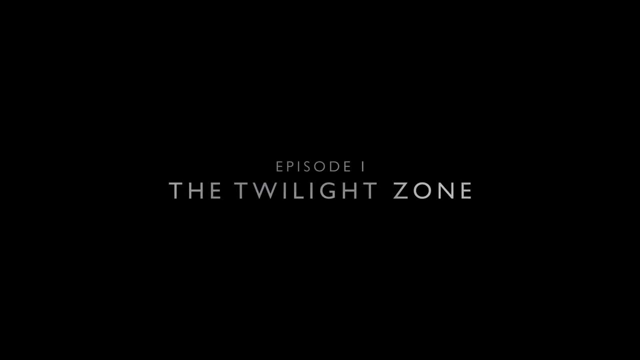 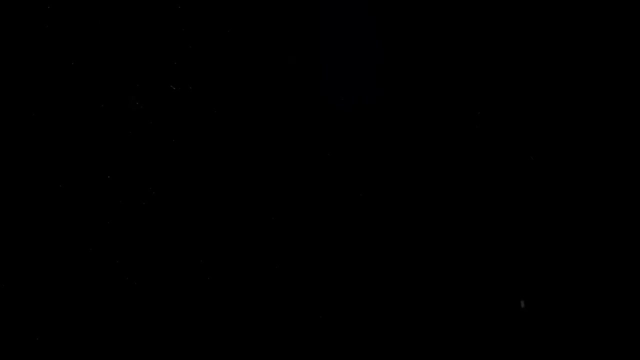 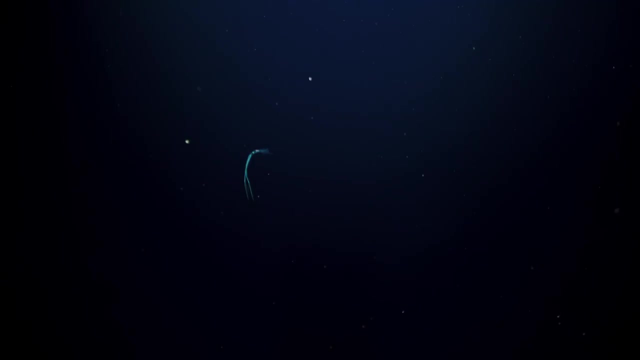 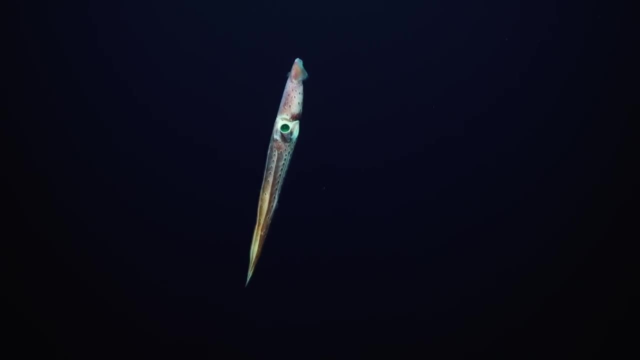 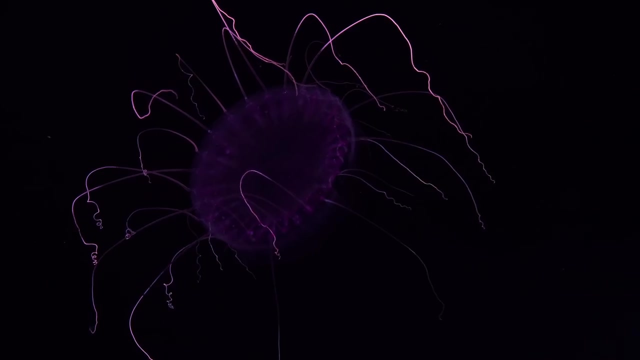 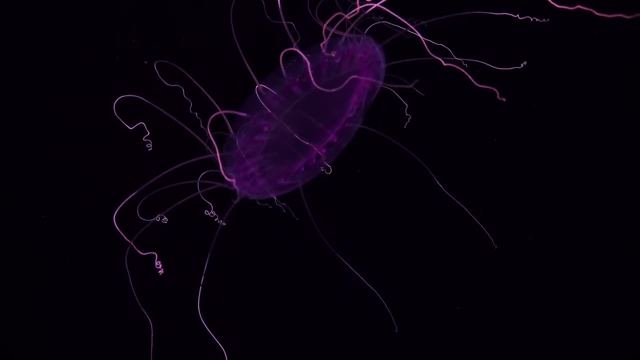 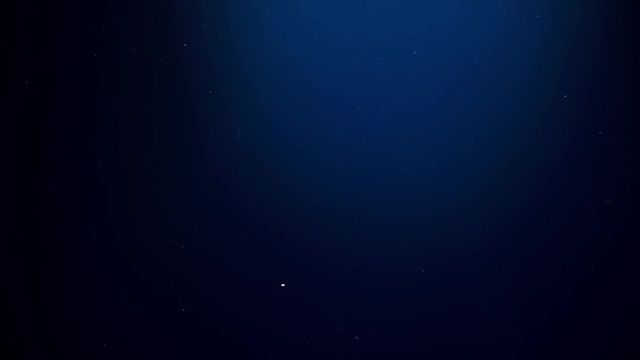 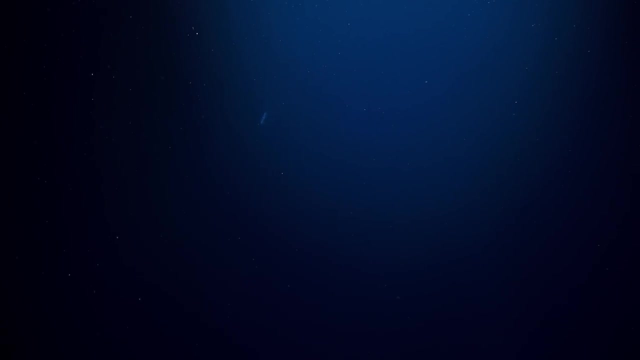 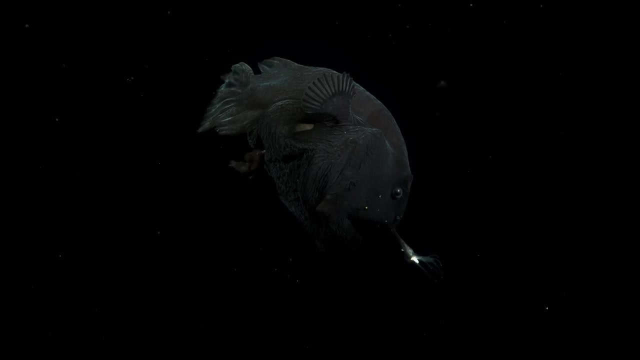 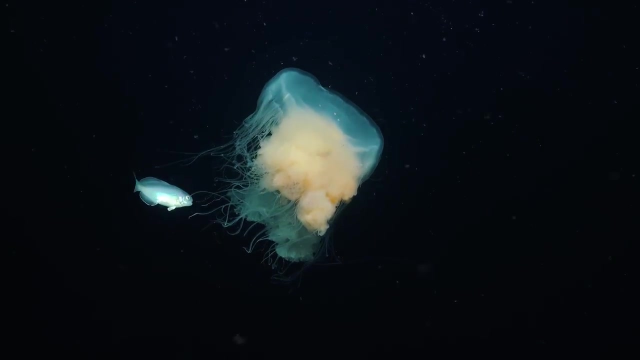 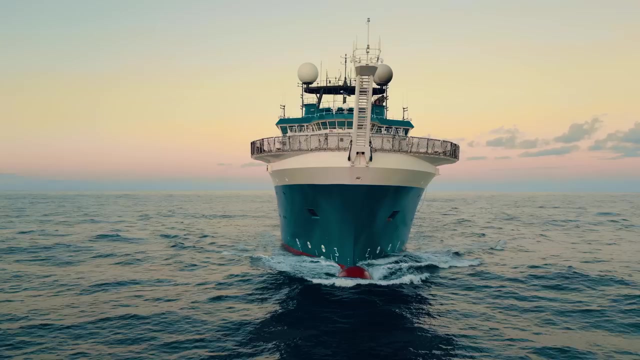 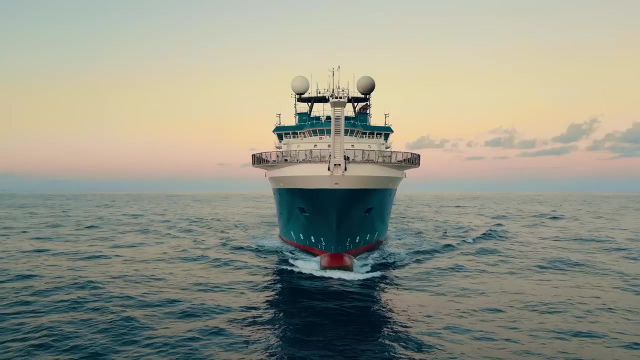 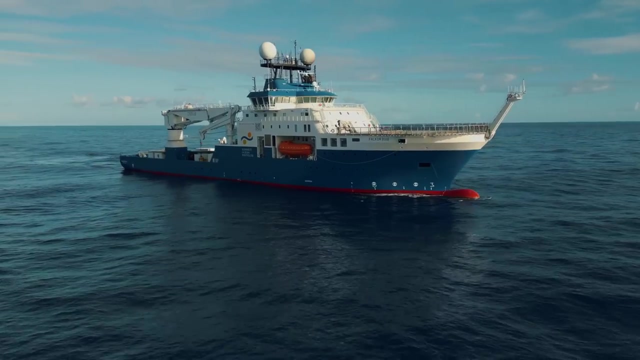 of zones based on depth and light levels, with each zone exhibiting its own challenges and hosting unique creatures that take on an array of unusual adaptations to survive. This is RV Falkor II, one of the most advanced research vessels in the world, on a mission. 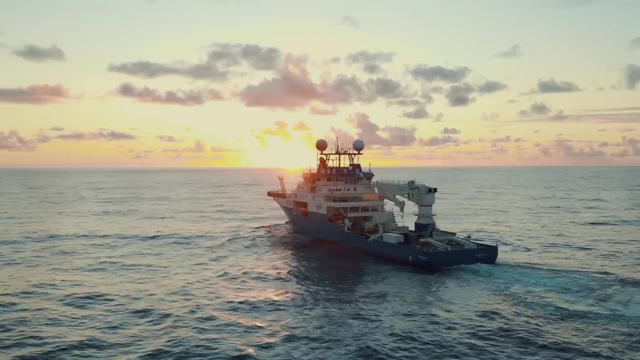 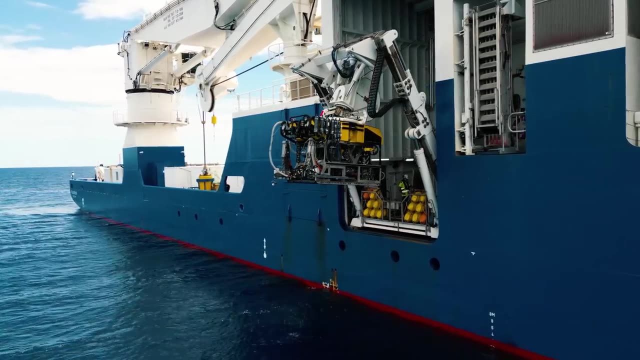 to discover our vast ocean ecosystem. Since 2009, the non-profit oceanographic research foundation Schmitt-Falkor II has been working on a new research project. Since 2009, the non-profit oceanographic research foundation Schmitt-Falkor II has been working on a new research project. 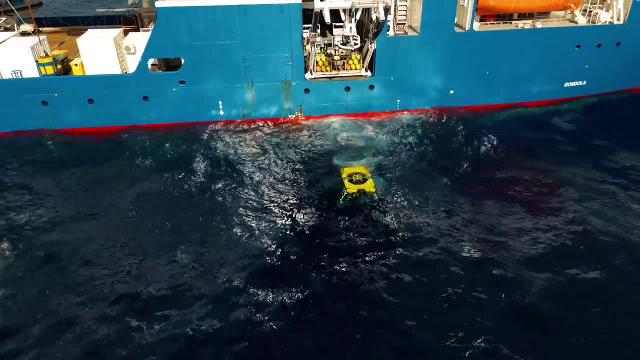 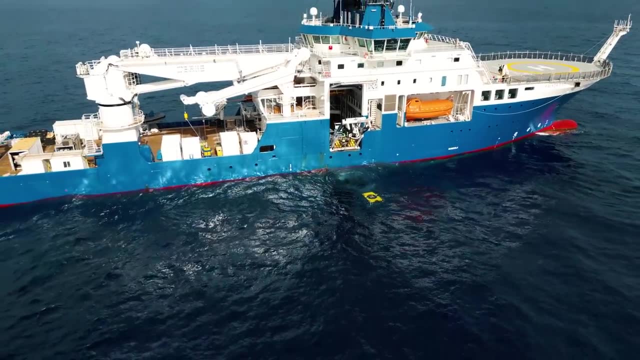 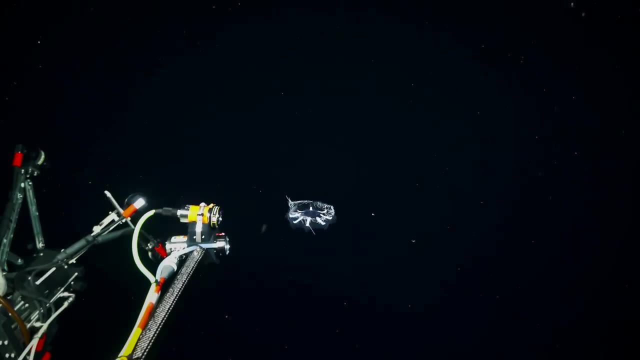 The Schmitt Ocean Institute have been exploring the worlds of the deep. Across more than 80 research expeditions, they have helped shed a light on the wonders lurking in the ocean's depths. Their remotely operated vehicle, Sebastian, has opened a window into this realm for all. 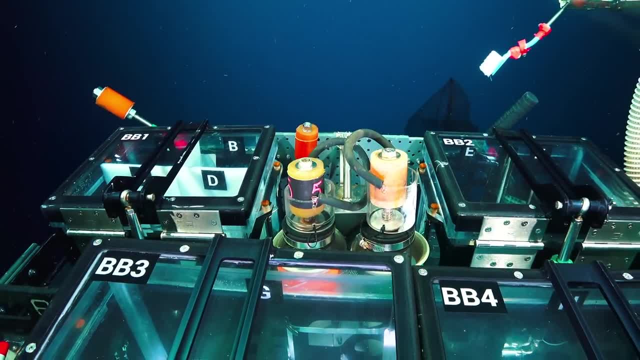 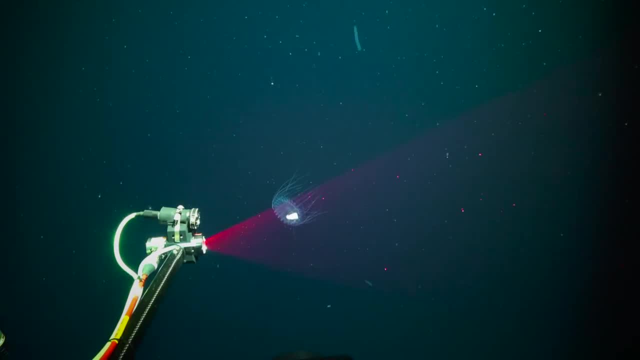 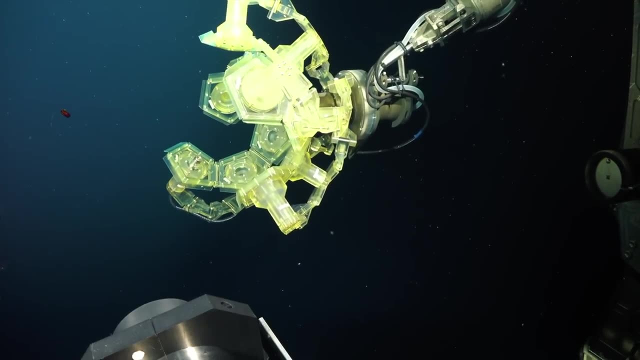 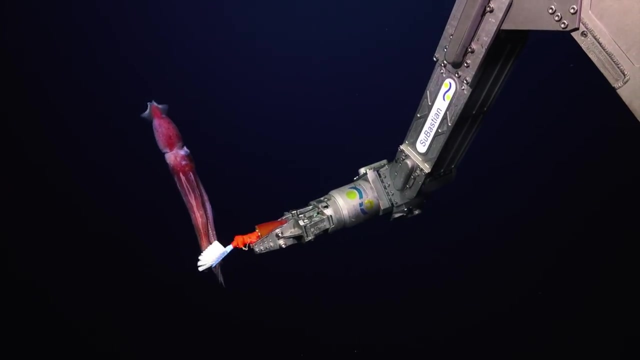 to see. Outfitted with a suite of sensors and a 4K camera, Sebastian is well equipped to explore the depths. Sebastian is capable of diving to 4,500 metres down in the sunless depths of the Midnight Zone. But in order to understand the unique conditions and challenges of life in deep sea midwaters, 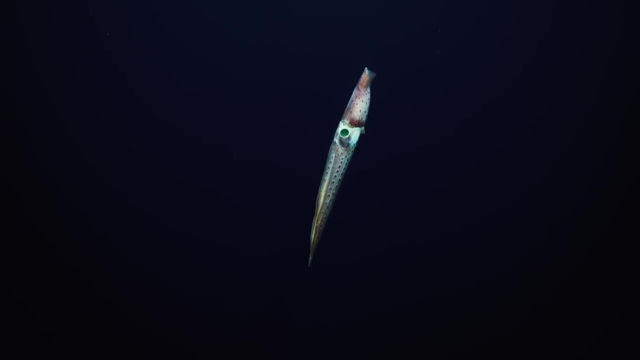 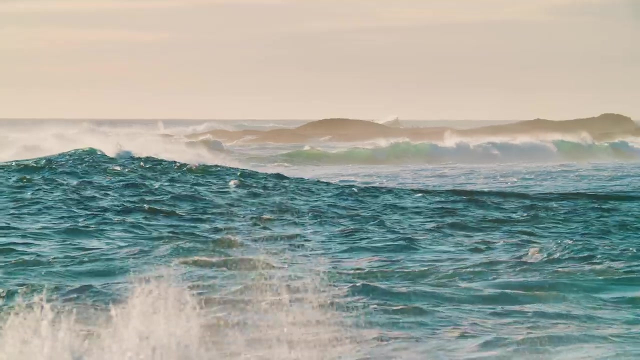 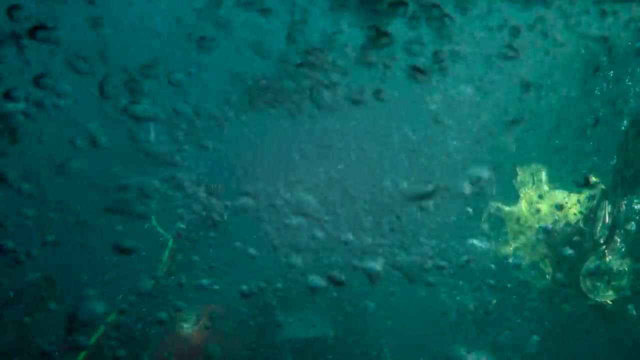 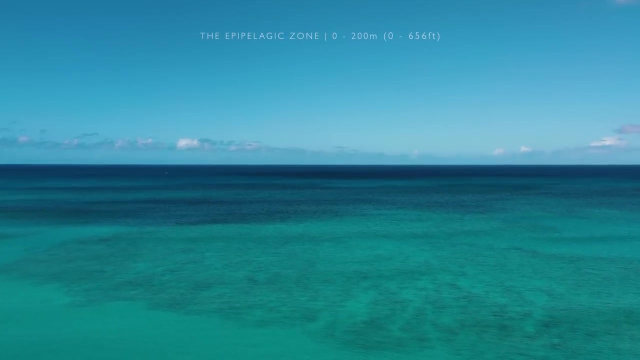 we have to begin at the surface Here. the epipelagic, or sunlight zone spans the upper limit of the water column down to a depth of 200 metres. It's a vibrant world. More than 90% of all marine life dwells here, and much of that belongs to the bustling cities. 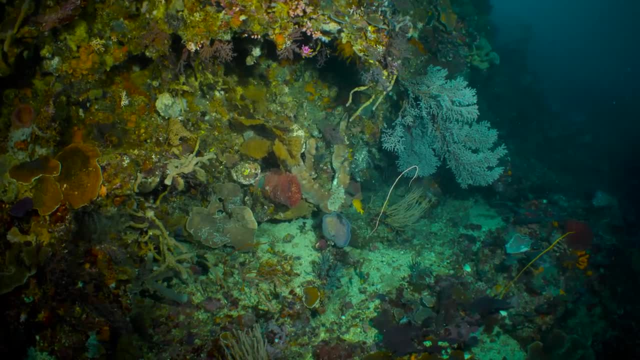 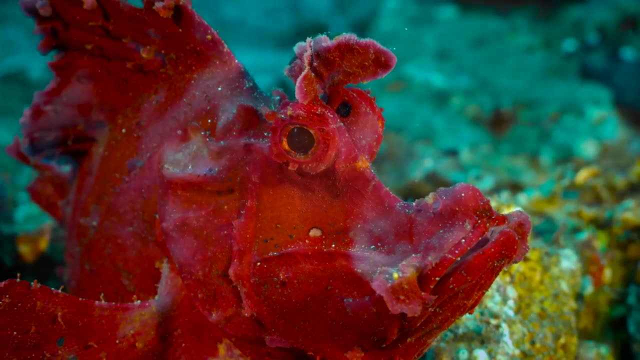 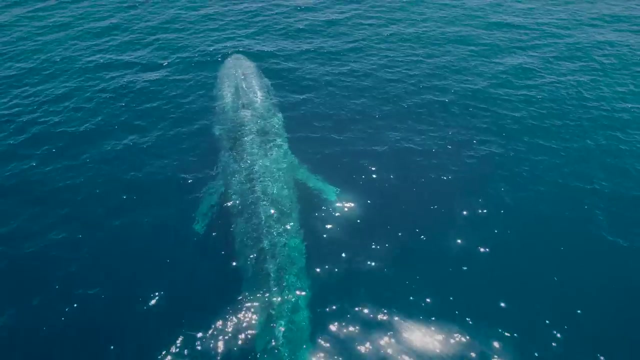 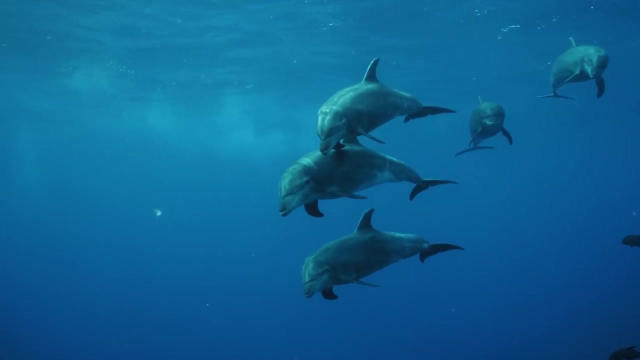 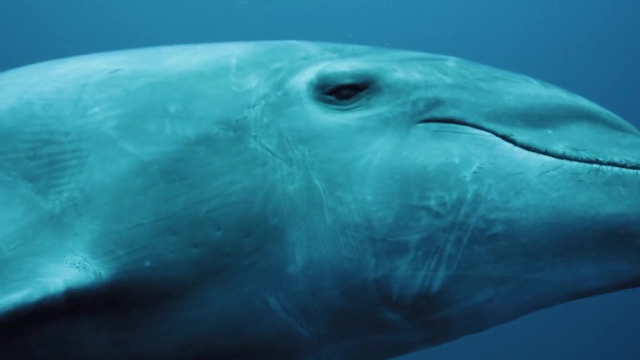 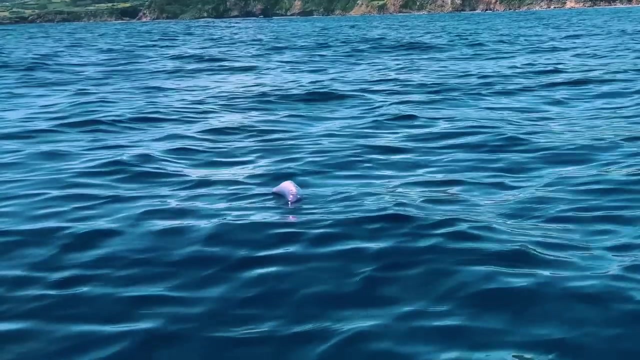 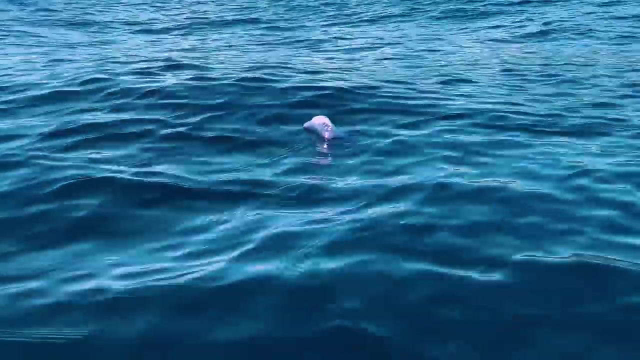 of coral in the tropics, Where food, Shelter And reproductive partners are not in short supply. Even out in the high seas, the sunlit waters host an astounding array of life. By developing a gas-filled float called a pneumatophore, the Portuguese man-of-war drifts 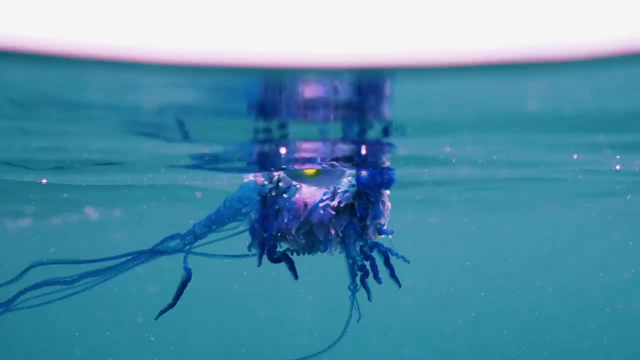 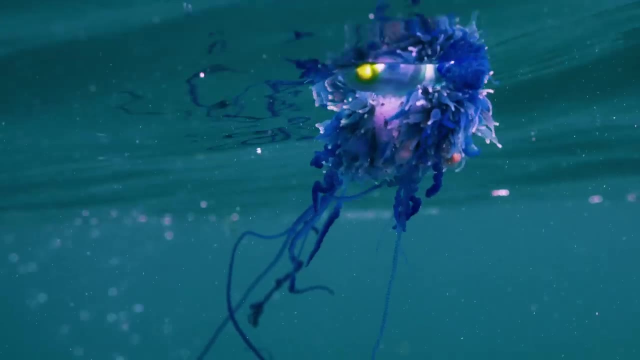 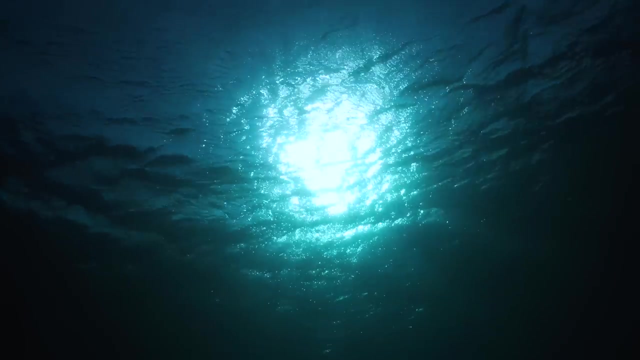 at the surface and uses wind to move, while downward-facing tentacles are used to feed. They are members of the Neuston, a community of floating animals that reside at the interface of air and water. Primary production is made possible near the surface by the rays of sunlight. 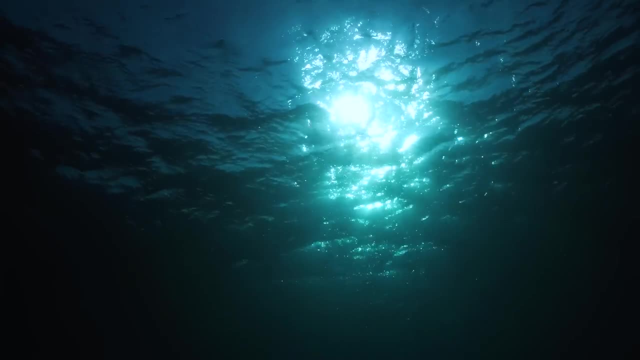 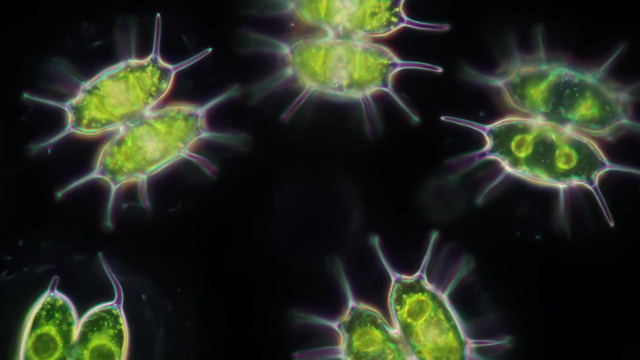 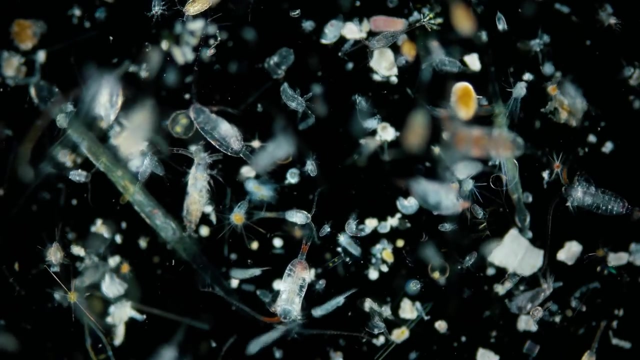 that filter through the waves. Microscopic plant-like animals called phytoplankton take on the role of producers, converting water and carbon dioxide into oxygen and glucose via photosynthesis. The biomass produced by this process supports all non-chemosynthetic life in the oceans. 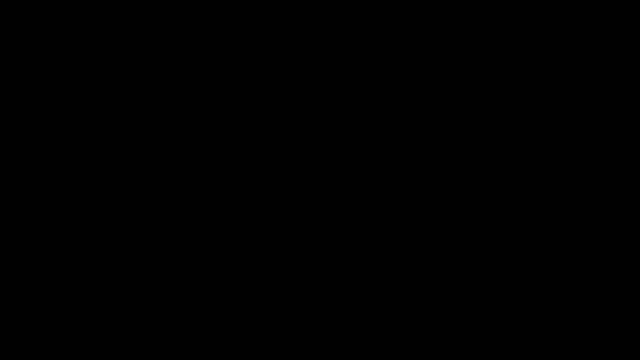 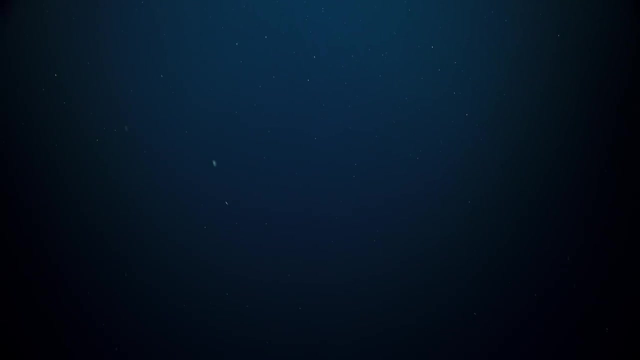 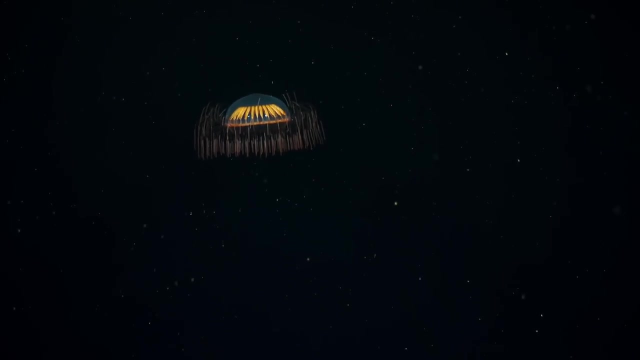 And without it, the depths below would starve, Dip below the epipelagic and we enter a world of gloom. This is the twilight zone, or the mesopelagic. From now on, we are in the deep sea, And already, at just below 200 metres, we are in the deep. 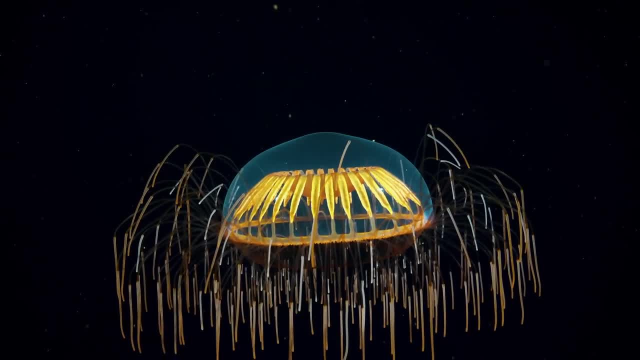 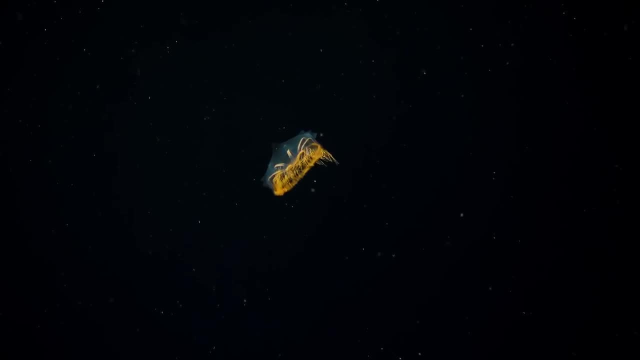 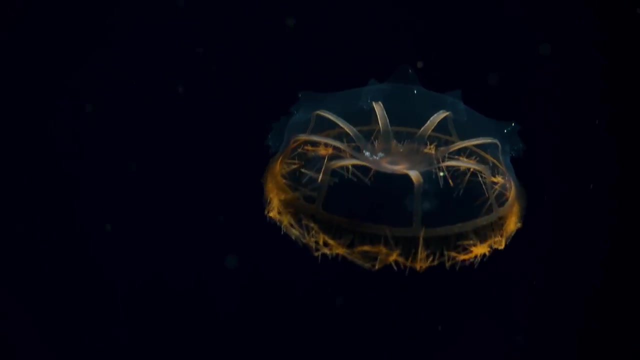 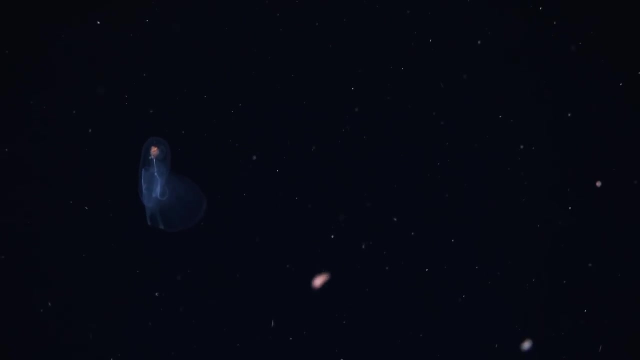 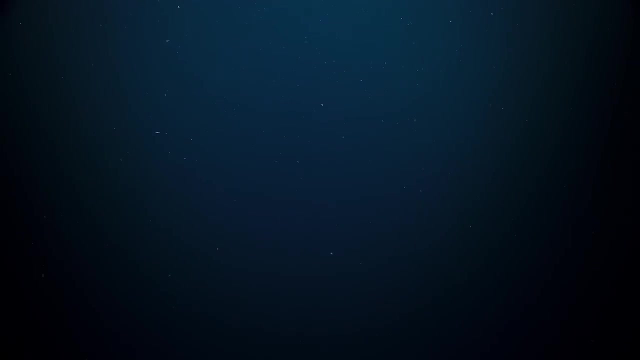 sea Survival is more of a challenge. There is not enough light for photosynthesis, and the great blooms of phytoplankton are absent. The only food source is a steady shower of faecal pellets and dead material- Organic particles called marine snow, gently sinking from the bustling world of sunlight up above. 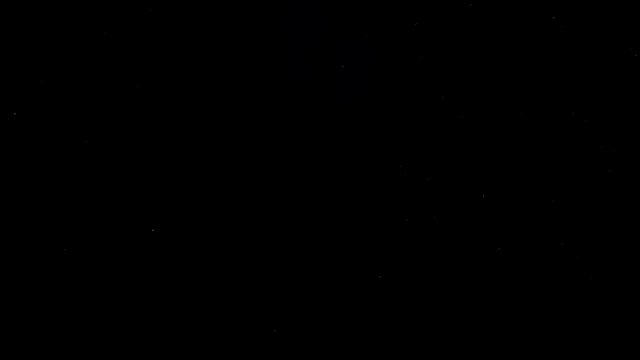 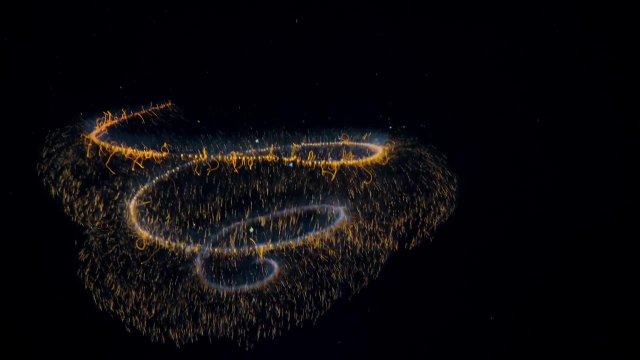 The presence of this marine snow gives rise to a unique niche that animals can exploit, and the great expanse of gloom brings forth the weird and wonderful. Many of these treasures are gelatinous zooplankton, swept by deep currents and unable to move. 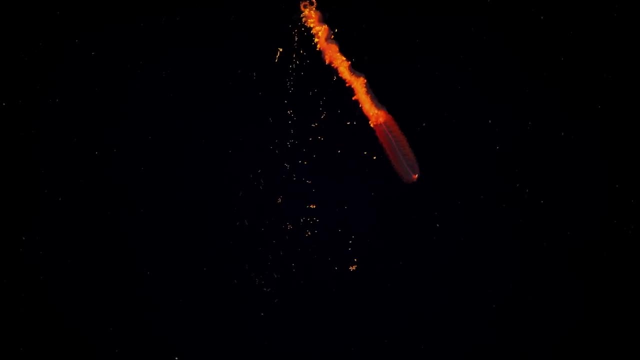 against them, A host of delicate nomads and a great number of animals are trapped in the deep sea and unable to move. against them, A host of delicate nomads and a host of delicate nomads are drifting through the expanse. 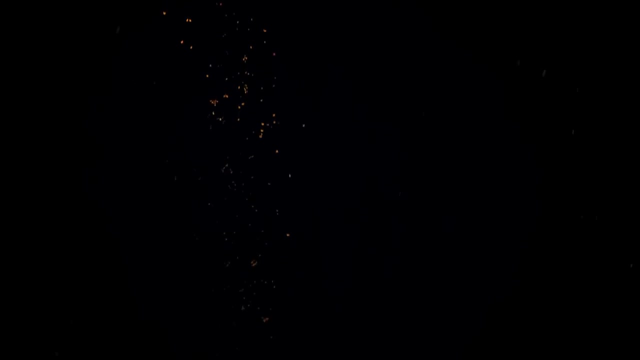 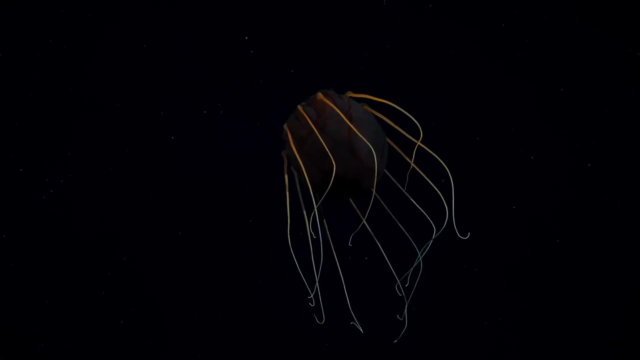 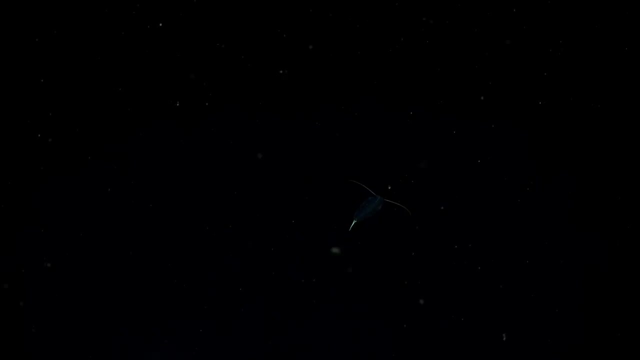 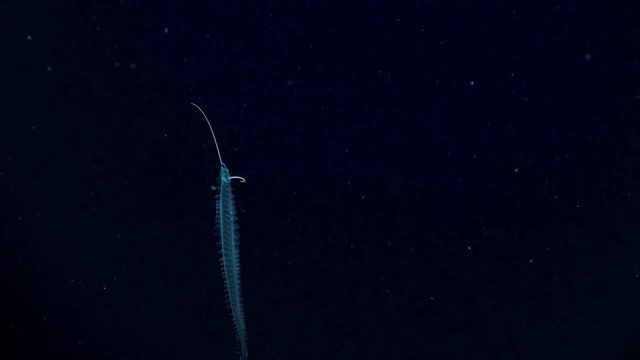 A few years later. the, The gossamer worm, or temopteris, is a segmented worm belonging to a group known as aphids, called polychaetes, meaning many bristles, And, unlike its cousin, the earthworm, it moves. 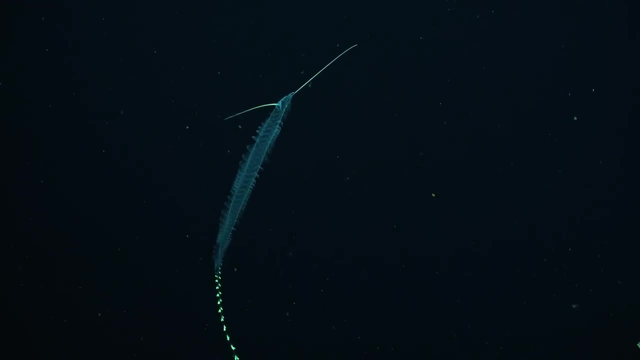 not through sediment, but through the open ocean. It undulates its bristles like the paddles of a canoe in order to swim and, after it's fed, the gut within its transparent body reveals the colour of its last meal. But this can blow their cover, since many 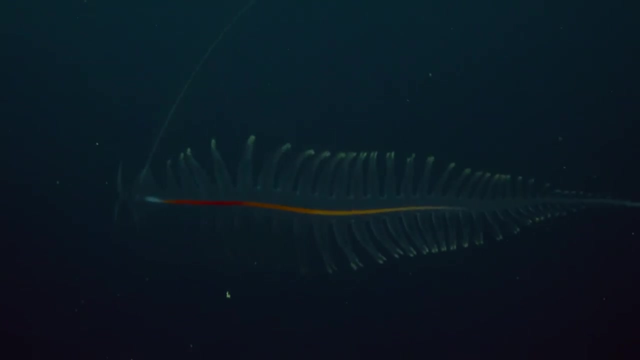 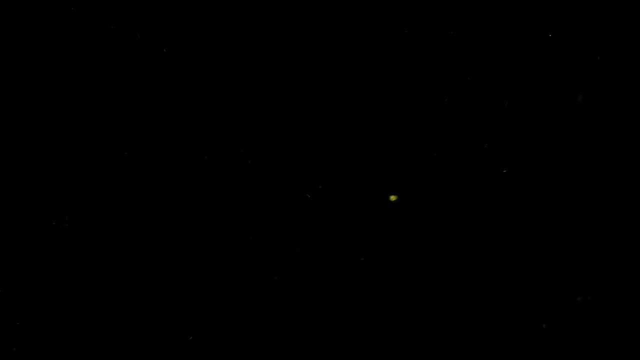 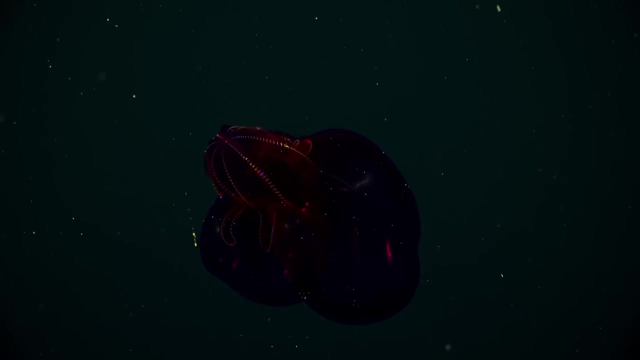 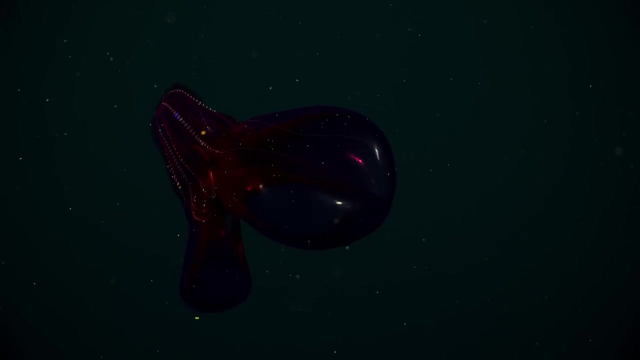 of the animals it eats are bioluminescent, creating light through a series of chemical reactions. There are others that have found creative ways to overcome this challenge. The bloody belly cone jelly undulates its hair-like cilia to attract prey reflecting light. to cast a rainbow shimmer, It takes on a deep red colour to make it look like 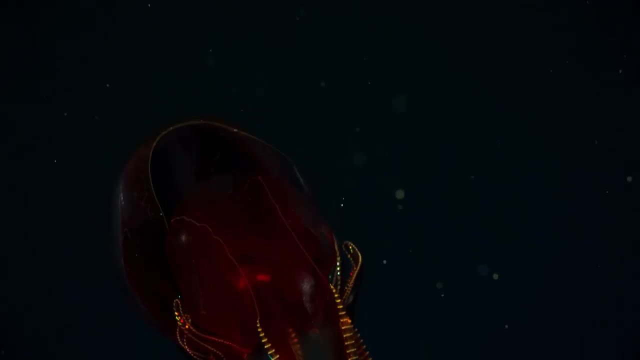 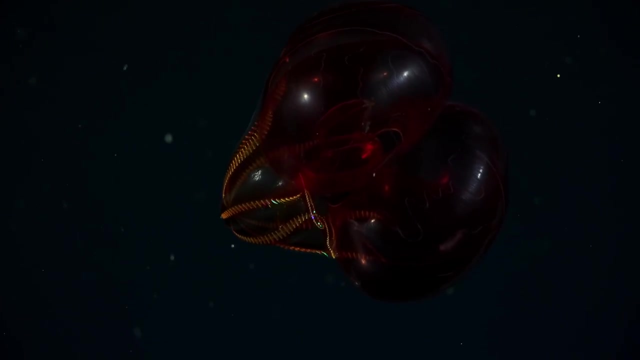 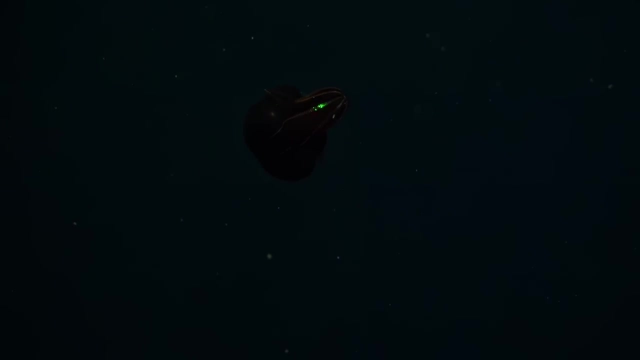 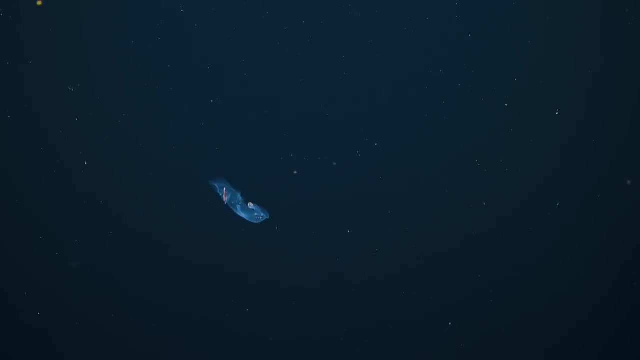 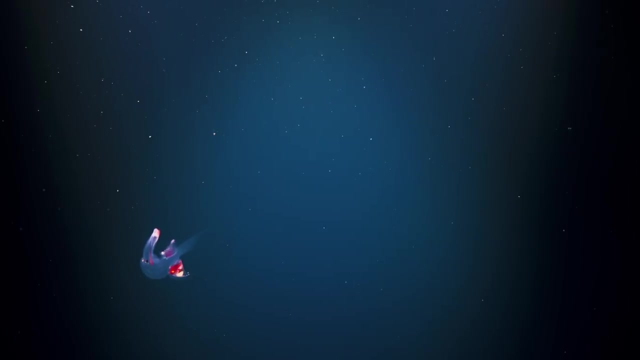 to blend in, since the wavelengths of red light do not reach the deep sea So, astonishingly, adopting a red colouration conceals the stomach and filters out any light being emitted by the prey within while they're digested. There are relatives of snails here too, like cardiopoda placenta, a rare pelagic gastropod. 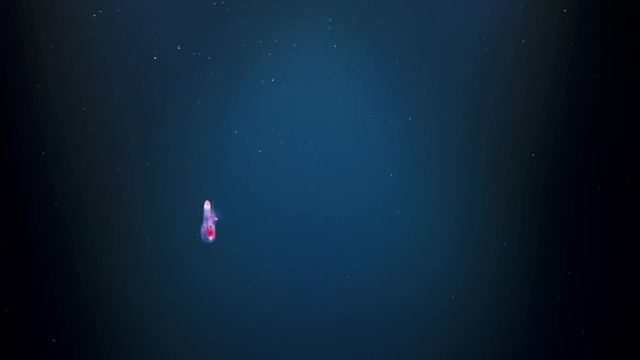 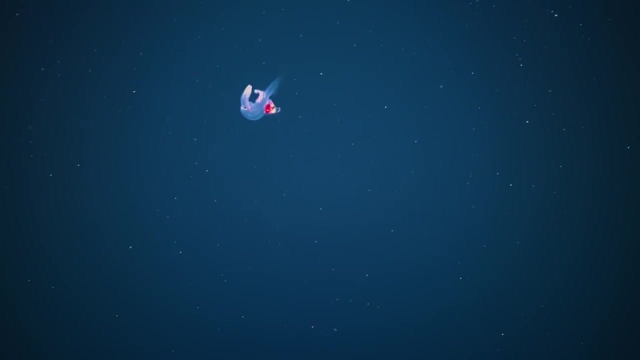 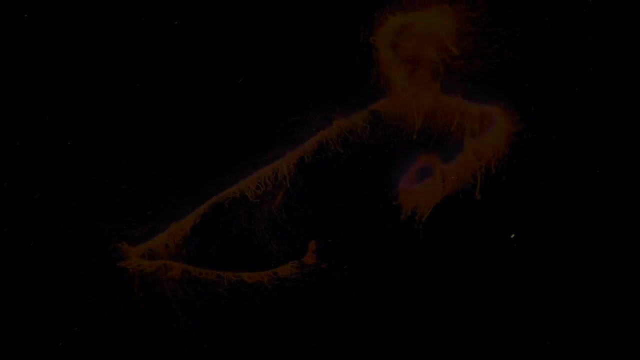 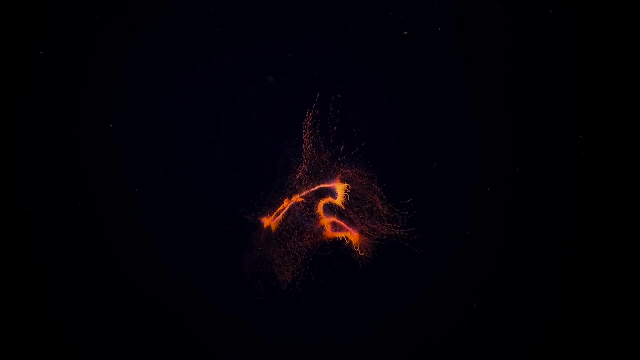 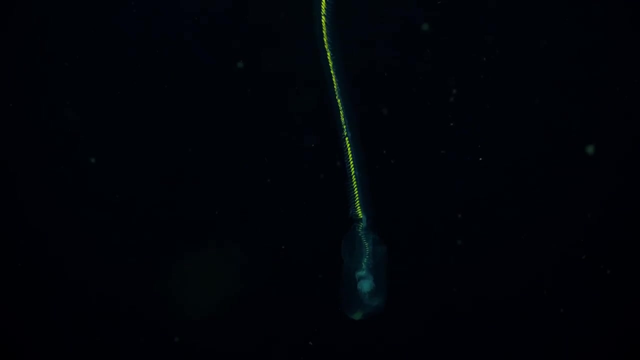 And another species, Carinaria japonica, with its large swimming fin, seems to prefer swimming upside down in search of prey. Siphonophores related to jellyfish are not one organism, but many. They are drifting colonies of tiny animals called zooids that work together and partition biological functions. 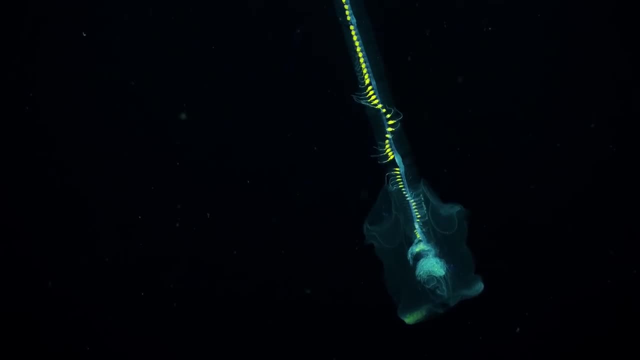 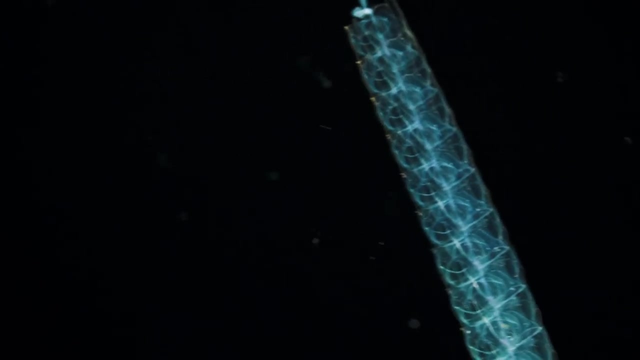 between different structures. Nectophores act as swimming bells assisting in propulsion, in much the same way as the umbrella of a jellyfish. They can also be used to create the colour of a jellyfish. Pneumatophores help with buoyancy And at the far end, gastro-zooids dangle tentacles. 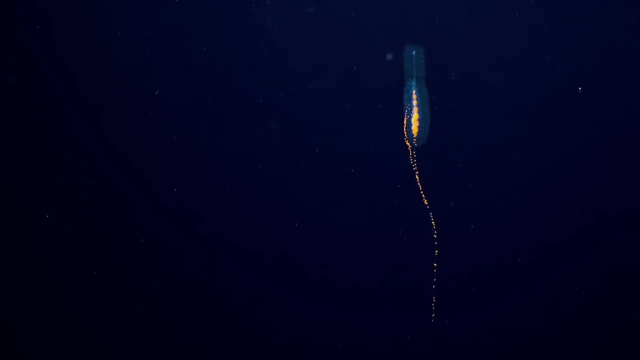 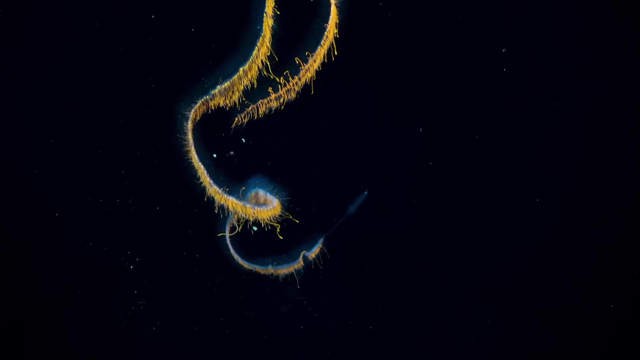 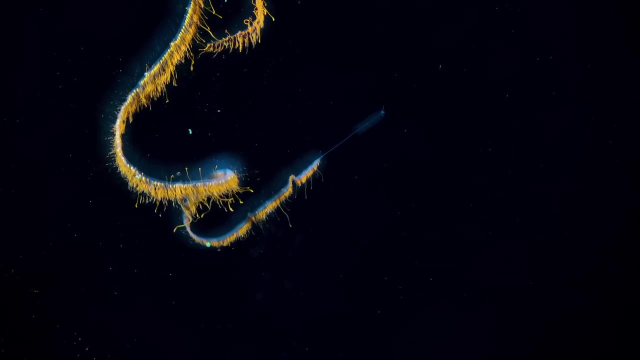 lined with stinging cells into the water, And it's their job to capture prey. The colonial way of life mirrors that of multicellular organisms, with the zooid structures seeming homologous to organs, but it gives the siphonophores a unique advantage: In most animals, damage 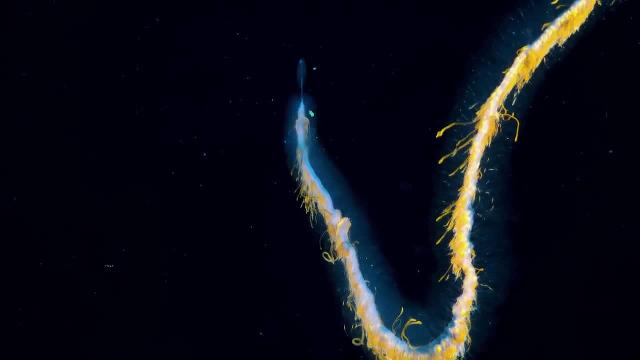 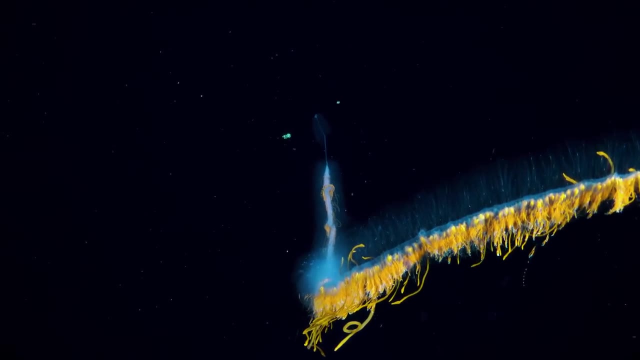 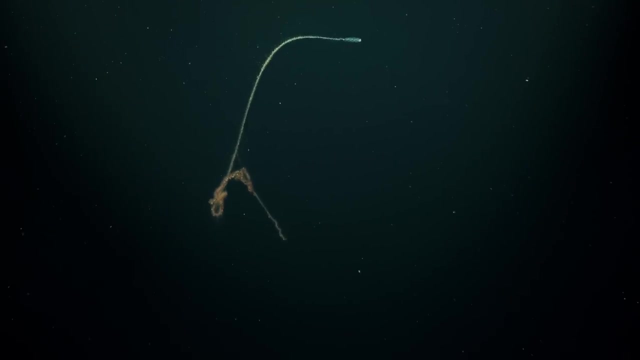 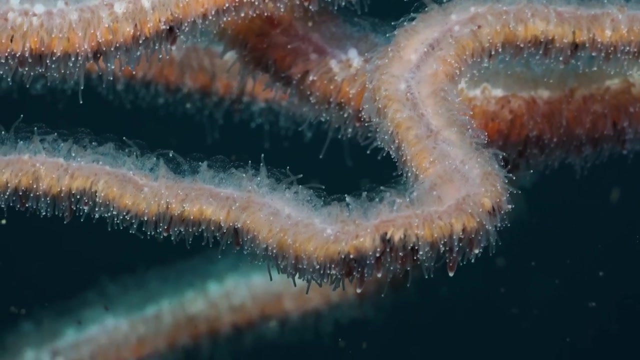 to one organ or physical structure is considered to be harmful, But if individual zooids become damaged, it's less likely to affect the entire colony. They repeatedly clone themselves and can become effectively immortal. This siphonophore belonging to the genus Apollimia is thought by scientists to be the 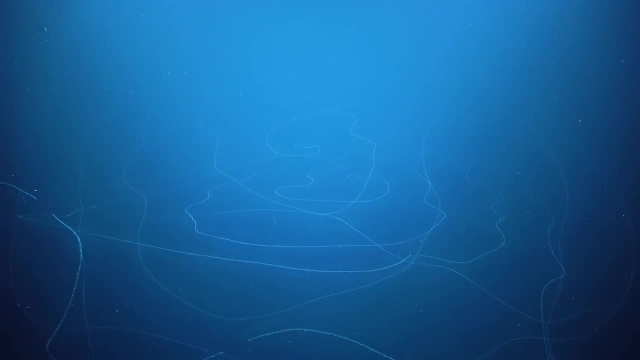 most dangerous species in the world. The genus Apollimia is thought to be the most dangerous species in the world. It is thought by scientists to be the longest animal that has ever been observed. Rough calculations based on the position of the ROV suggest that it reached 50 metres in length- Longer even. 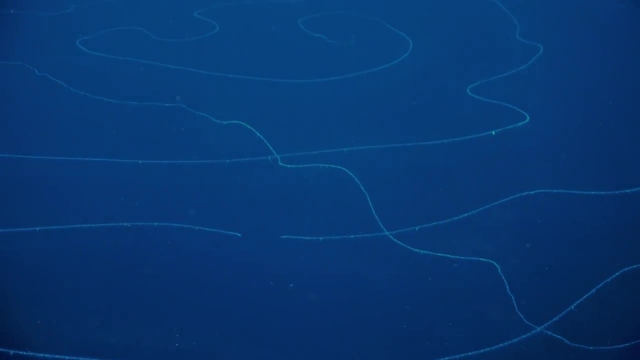 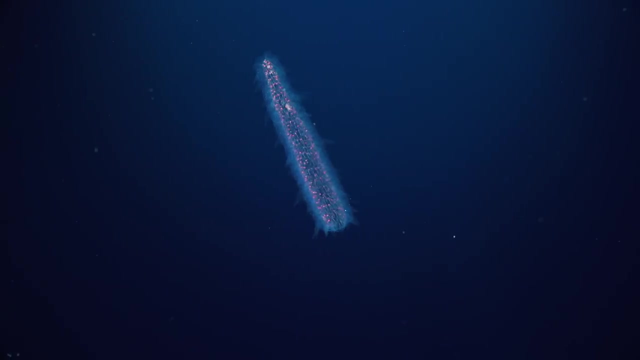 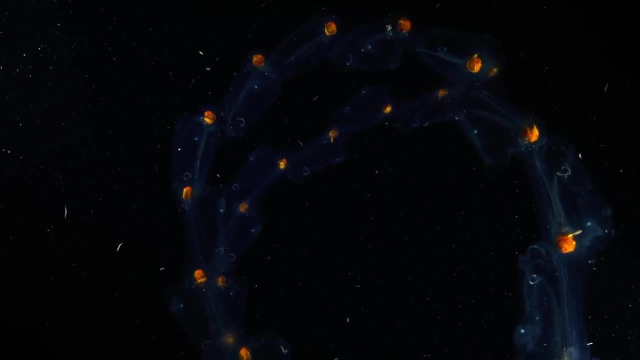 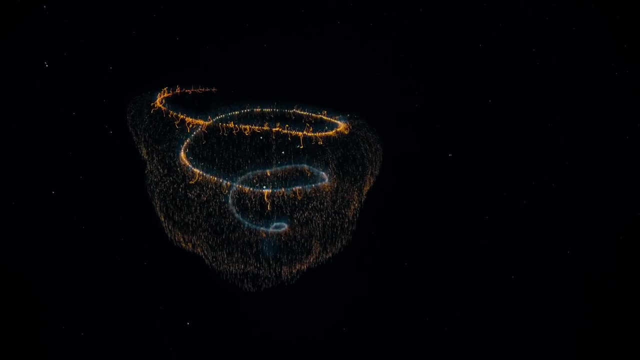 than a blue whale. Many tunicates are also colonial, like pyrosomes And floating, necklace-like salps. All of these plankton examples can be classified as holoplankton, meaning they are permanent members of the plankton throughout the entirety of their life cycles. 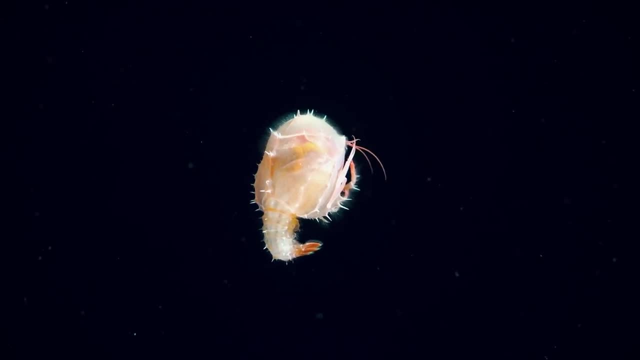 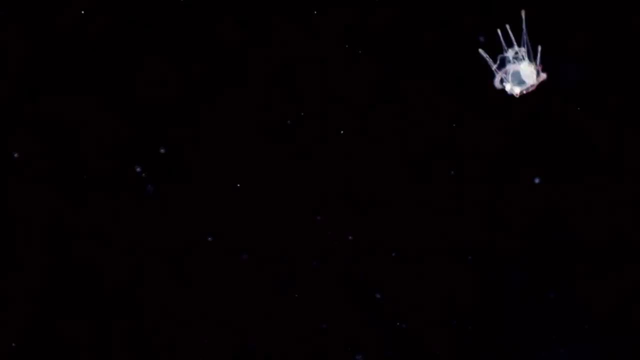 Meroplankton, on the other hand, are only planktonic temporarily and are typically the larval stages of fish or species that spend the adult stages of their life cycles in the benthos far below. The plant is known as the plantinus and is known as the plantinus of the plantinus. 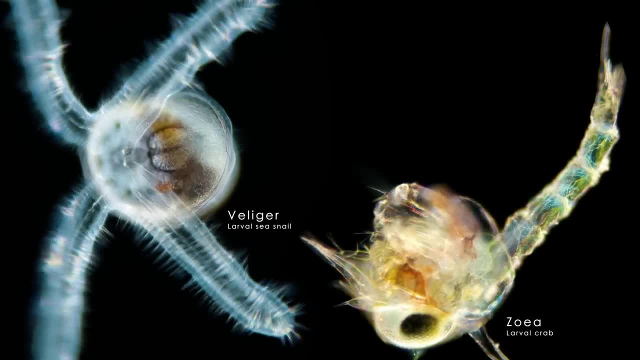 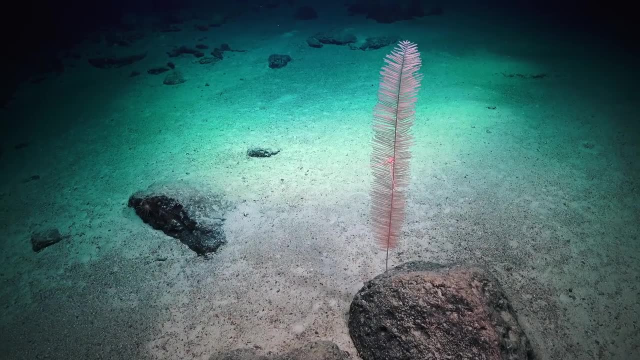 It is known as the plantinus of the plantinus. and is known as the plantinus of the plantinus, Like molluscs, crusta, ogóle and echinoderms, who will one day settle on the seafloor. 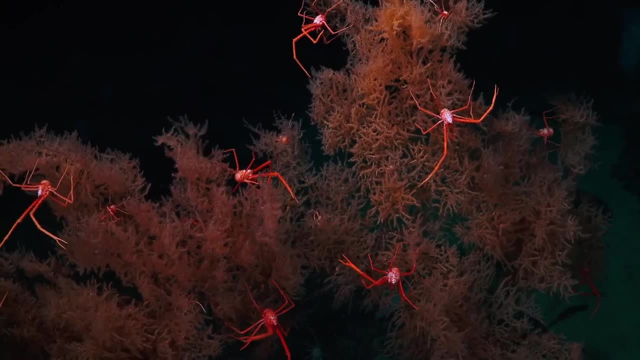 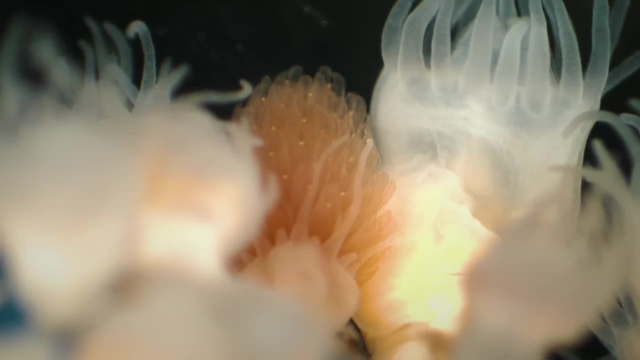 For some animals the reverse is true, and it's the larval stage that's cessal. Enter verse 8, The life cycle of many jellyfish begins in the sea. After 235 years, living mouthes and gills of a presented mottled one. 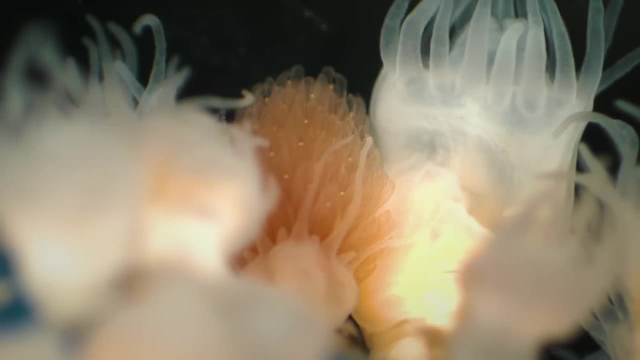 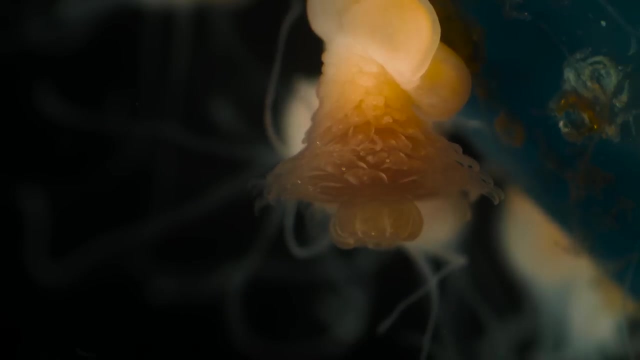 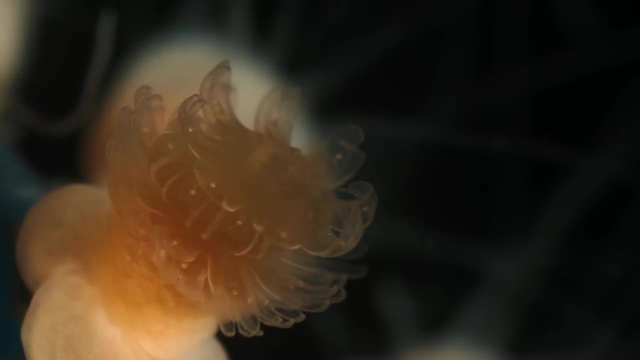 So manyjam jellyfish begins with a polyp form on the seabed Planular larvae, settle and develop into a scyphistoma, before asexually reproducing to create a stack of developing juvenile medusae called a strobila. These juveniles bud off one by one and develop into pelagic adult forms of. 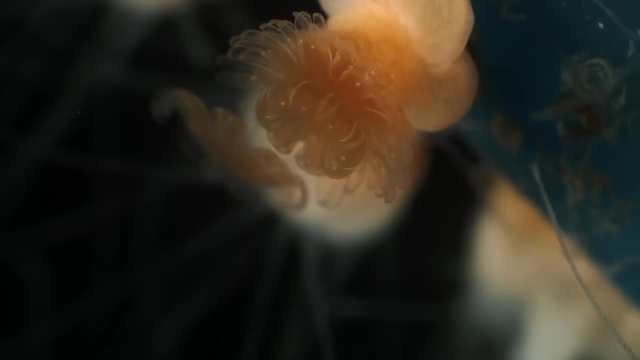 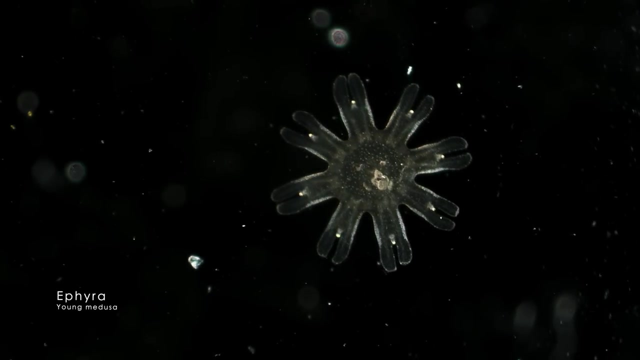 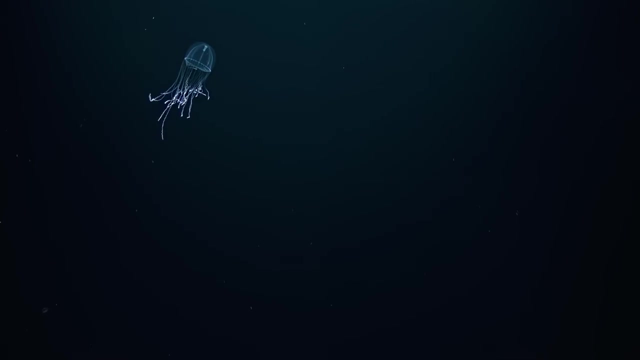 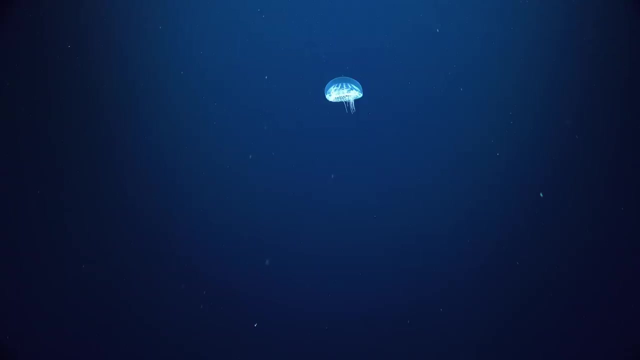 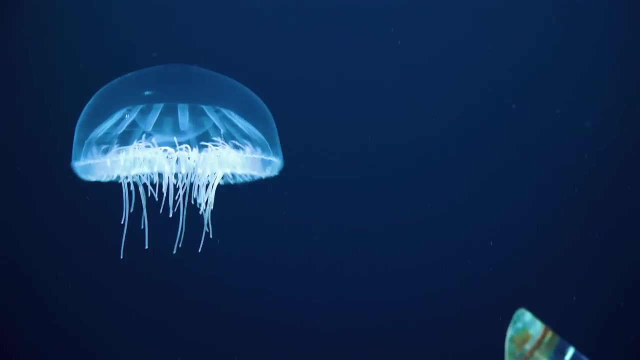 jellyfish, And the midwaters are full of them, But since the seafloor is so far away, many jellyfish here lack a polyp stage altogether and complete their entire life cycles in the water column. Some host the young larvae within their bell as they develop. 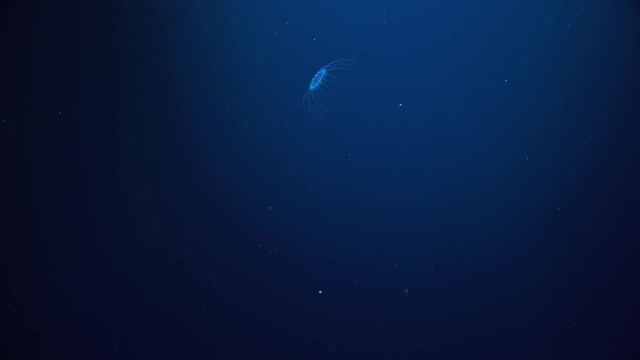 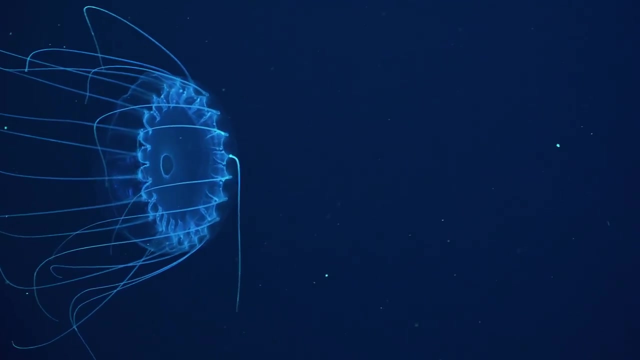 The dinner plate. jelly swims with its tentacles extended forward, A technique that allows them to stealthily sneak up on larger prey without startling them with large water movements. Remember, in all the footage we're seeing the lights of an ROV are illuminating the 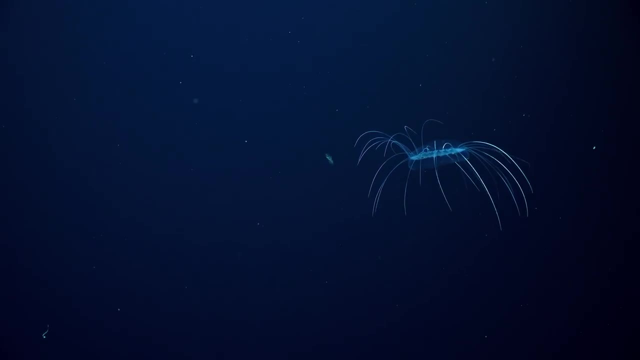 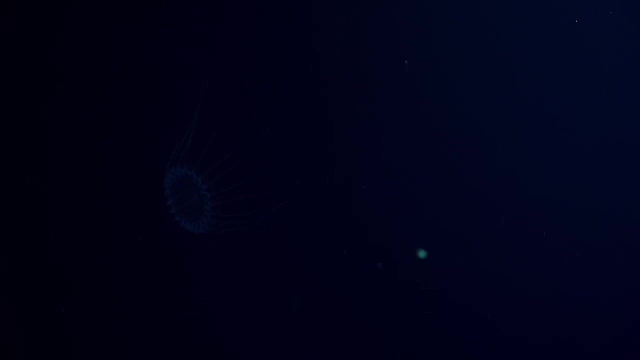 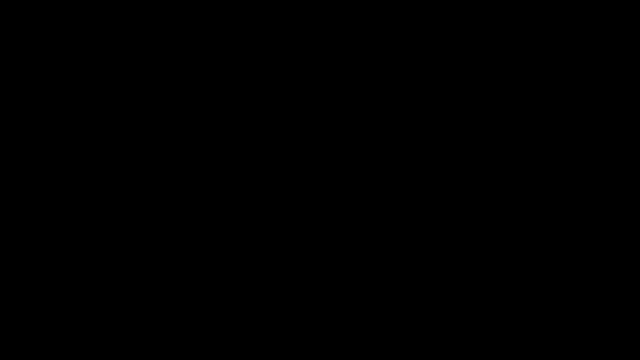 animals and the surrounding waters, so it's hard to imagine just how difficult it would be for prey to avoid slow-moving predators like this one in the gloom. There are also active swimmers- Nekton rather than plankton- And a great number of them are. 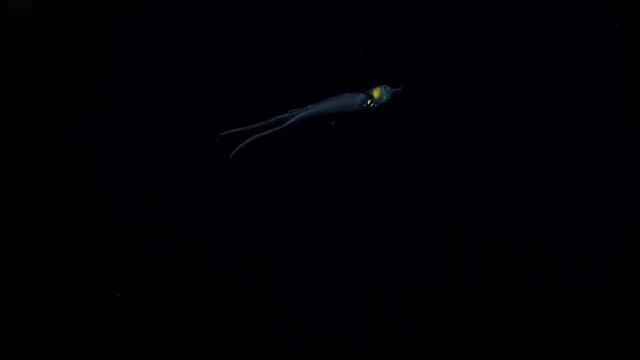 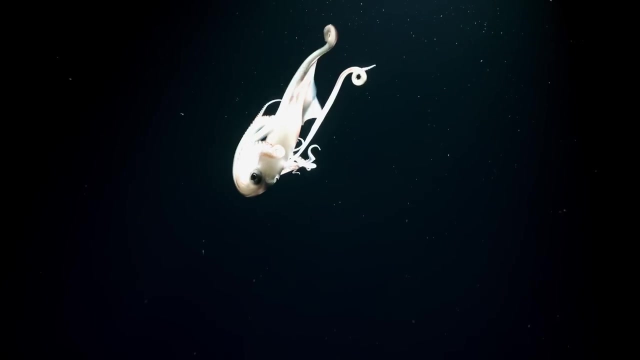 cephalopods, The squid, octopus and cuttlefish. The largest and most intelligent of the ocean's invertebrates. The most intelligent of the ocean's invertebrates. The largest and most intelligent of the ocean's invertebrates. The largest and most intelligent of the ocean's invertebrates. 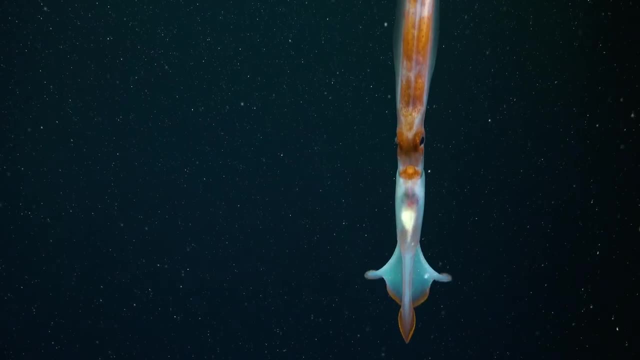 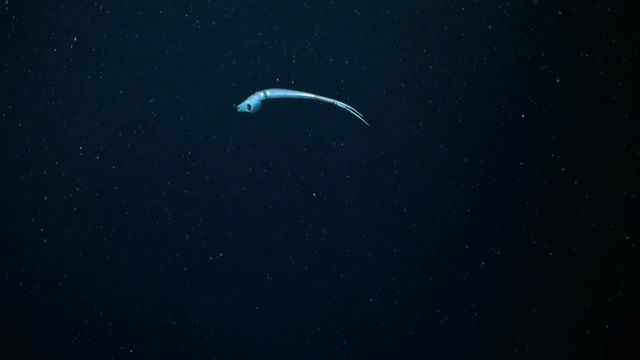 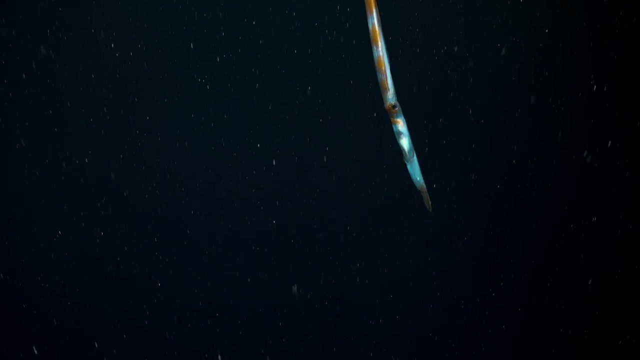 They are mollusks related to snails and bivalves, but their basic body structures are modified and specialised to make the most of life in the open ocean. The mantle has become streamlined, and a modified foot serves as a set of eight or more. 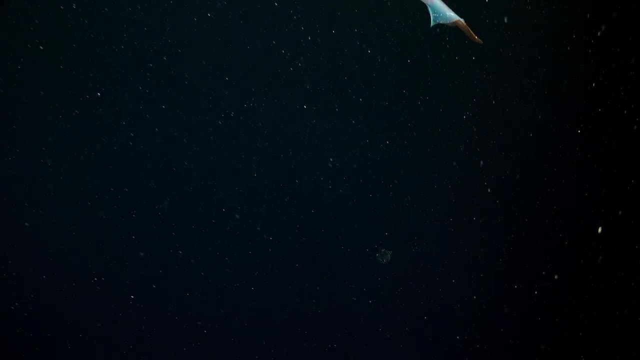 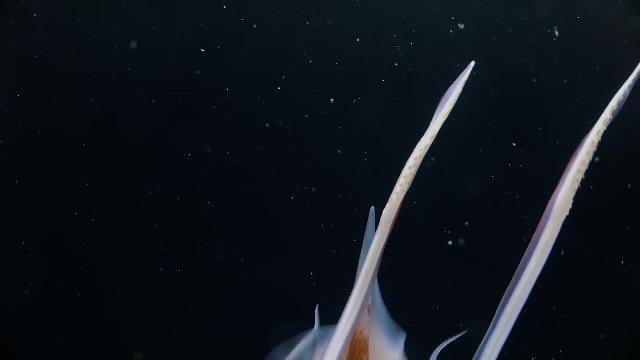 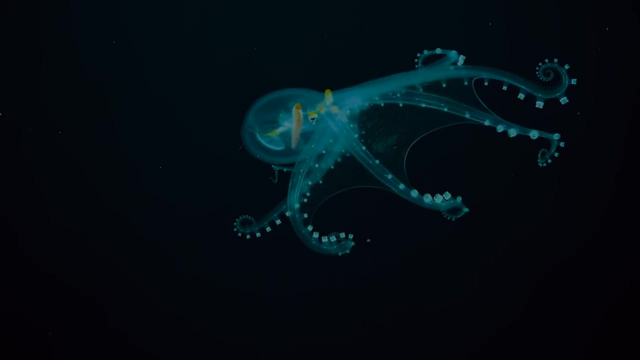 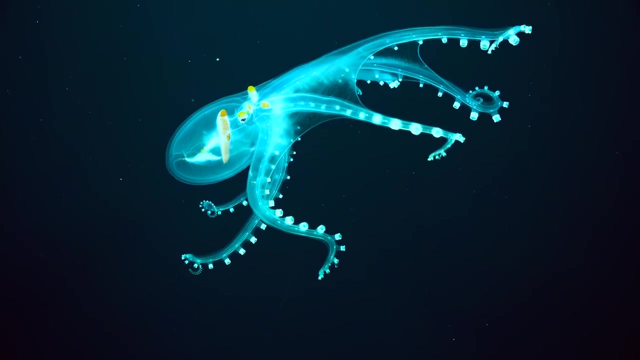 arms. At 650 metres down, we find an octopus that is almost entirely see-through. This is a glass octopus and it is around 40 centimetres long. The eyes of the octopus are believed to defend themselves against杯. 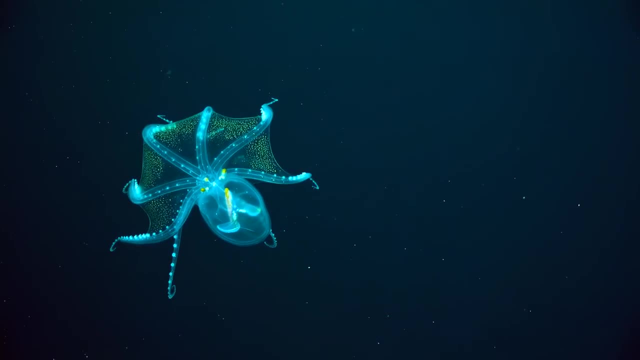 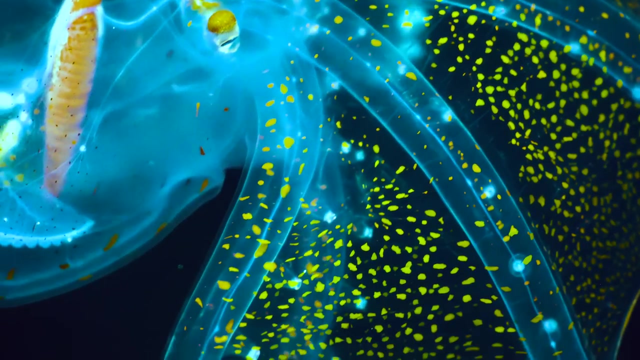 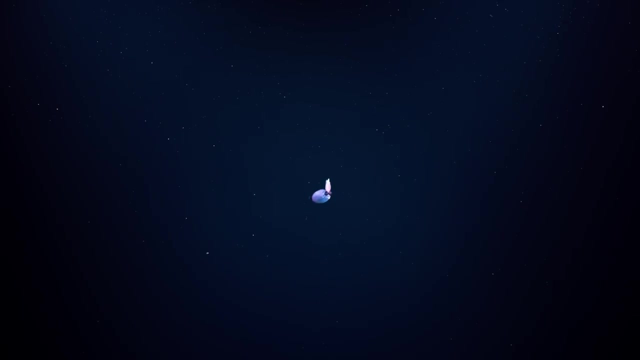 water happy Boston fluid. the eyes of the octopus have Si studying whole body fluids it services. Their eyes are one of only a few structures visible within its glass-like mantle. The glass squid with its bulging eyes has also developed a body that is transparent. 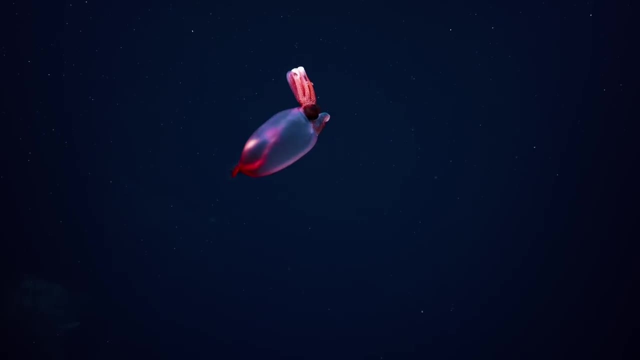 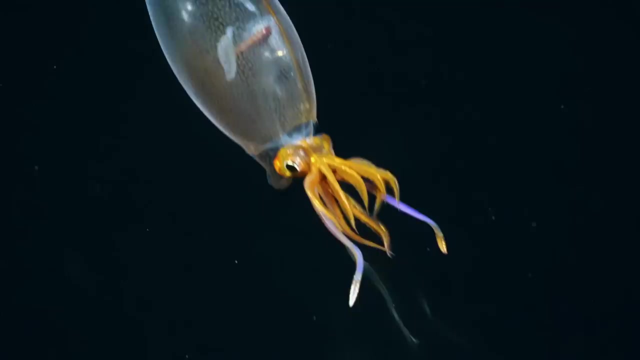 Most of the time, When it suits them, they change the colour of their skin and fill their mantle with ink to turn deep red. Their ink also contains ammonia, which is lighter than seawater and allows the squid to remain buoyant. See-through animals are more abundant in the deep ocean than anywhere else. 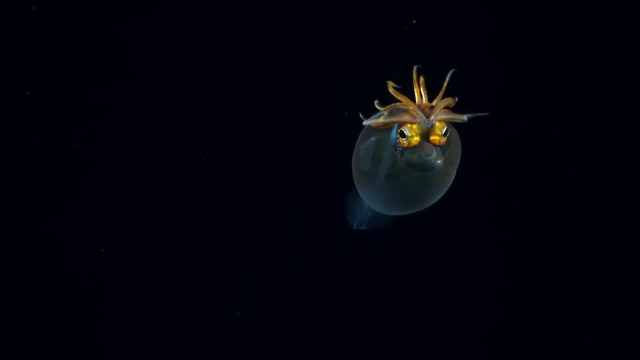 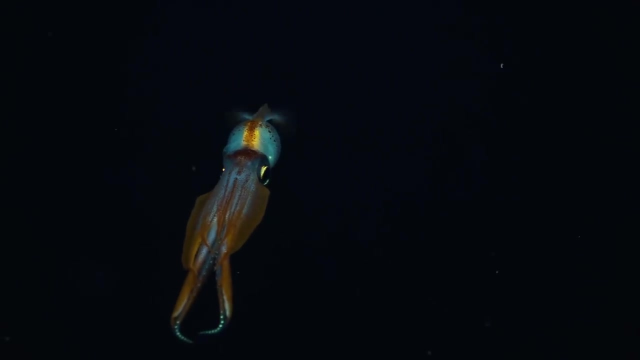 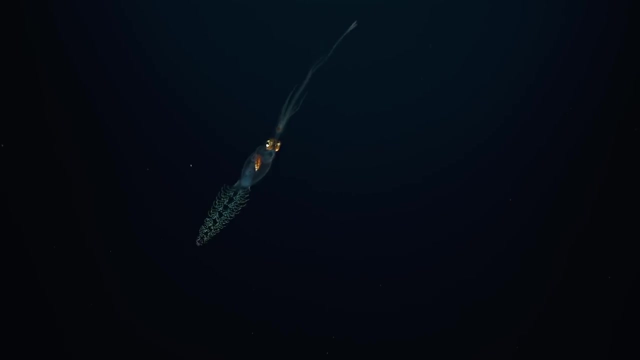 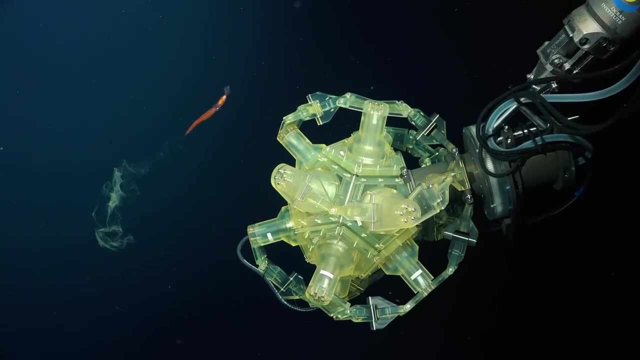 In the depths, there are no harmful UV rays to necessitate cell pigmentation as a way to protect them from solar radiation. Inking is also used for defence When spooked squids flee quickly and leave behind a shroud of ink in the form of a cloud, rope or other shape resembling ghostly apparitions in the gloom. 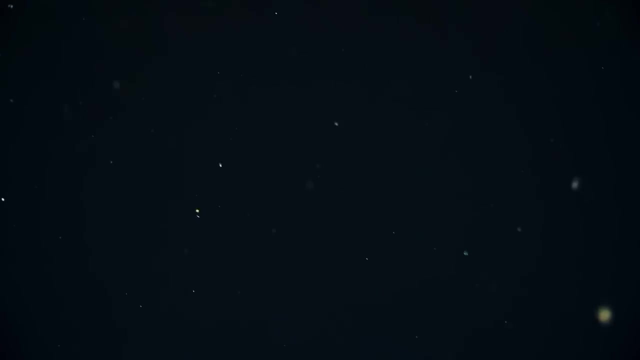 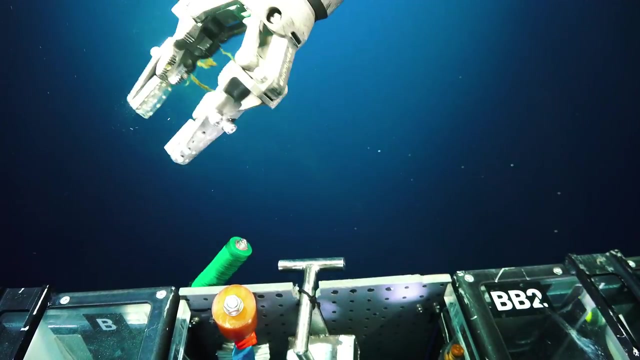 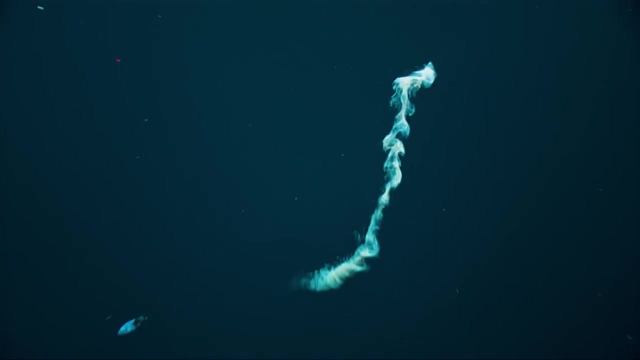 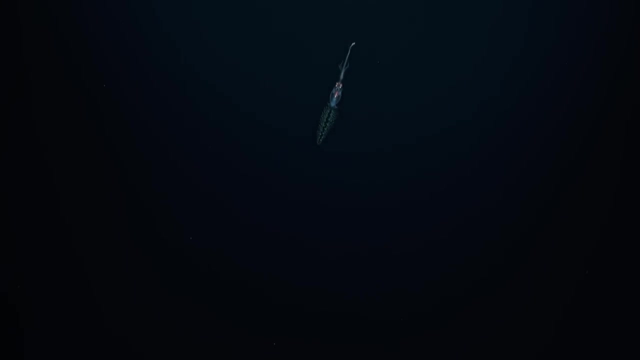 The ink masses are thick. They are thought to be animal look-alikes, dubbed pseudomorphs, and they serve as a decoy. Some look like comb jellies or jellyfish, Others resemble siphonophores. In some cases, it may be advantageous for the squid itself to look like another animal. 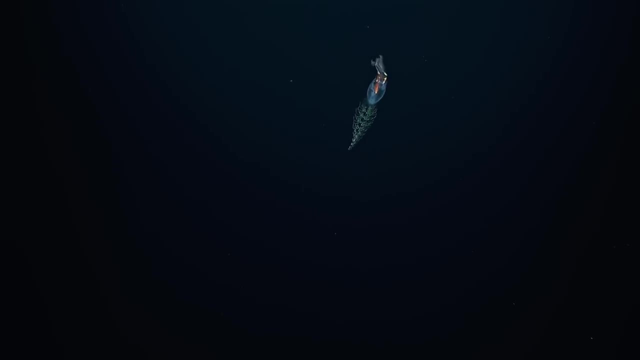 Juveniles of the sword-tailed squid were observed mimicking siphonophores of the genus Nonomia. When young, they possess ornate tails that double the length of their bodies and seem to copy the shape and colours of their gelatinous neighbours. 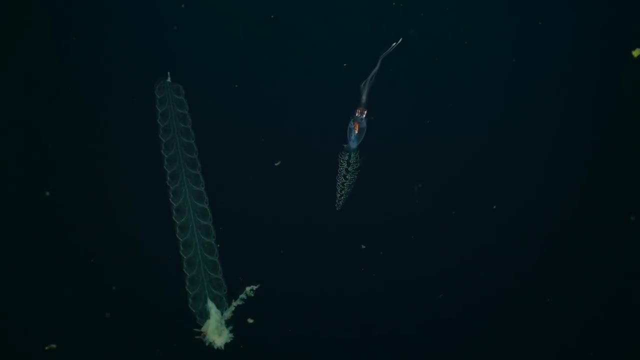 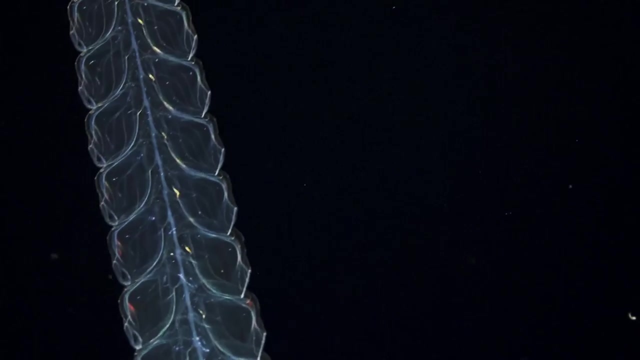 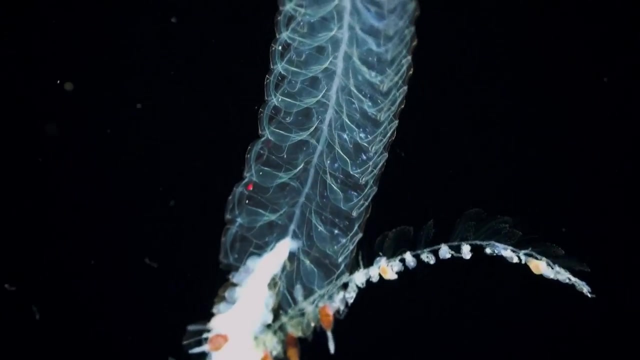 They even position their tentacles in such a way that makes the deception more convincing. Siphonophores are not a dense source of food. They are mainly water, and this, coupled with the stinging cells that line their bodies, means they are not on the menu for many animals. 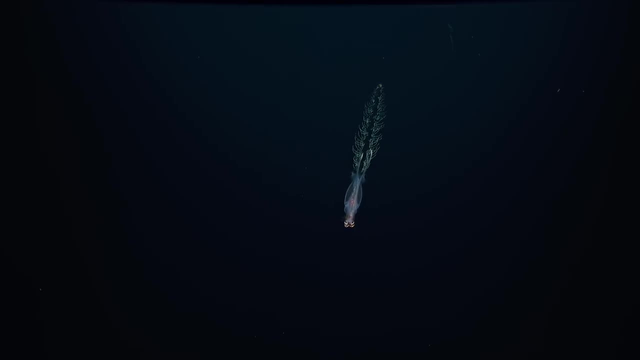 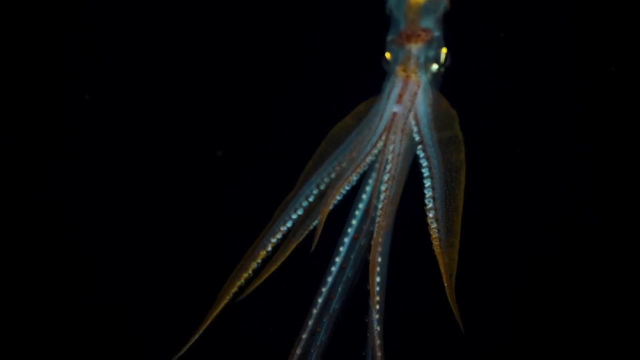 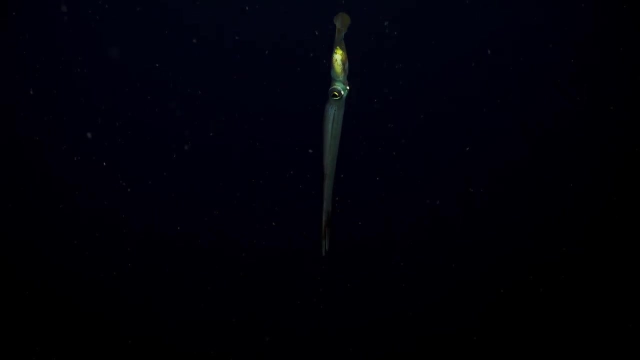 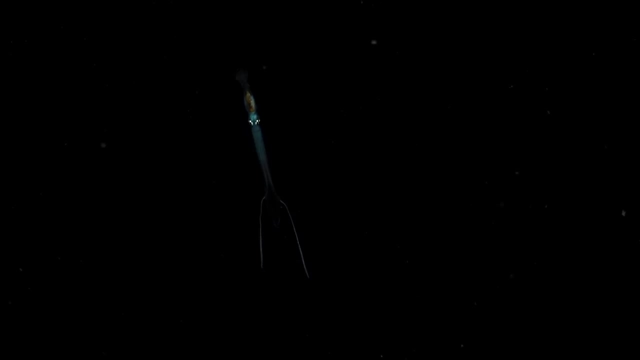 And so the juvenile sword-tailed squid appear unpalatable to predators, who mistake them for the siphonophores. In their adult form, Chira-toothed squids become impressive hunters. The two feeding tentacles are expelled rapidly, tipped with clubs at the end lined with suckers for grabbing prey. 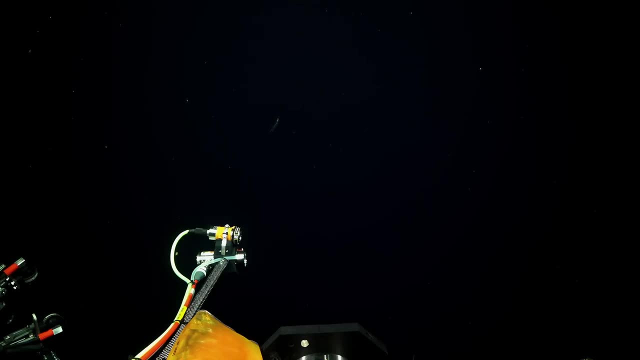 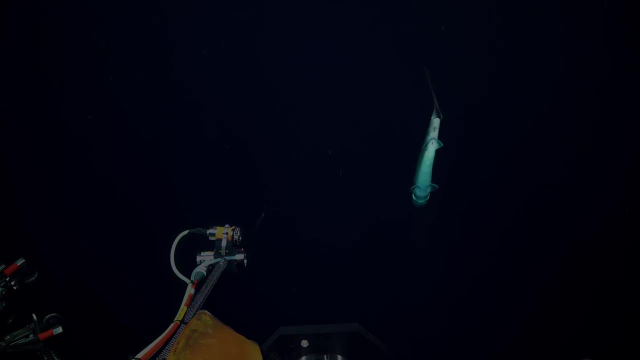 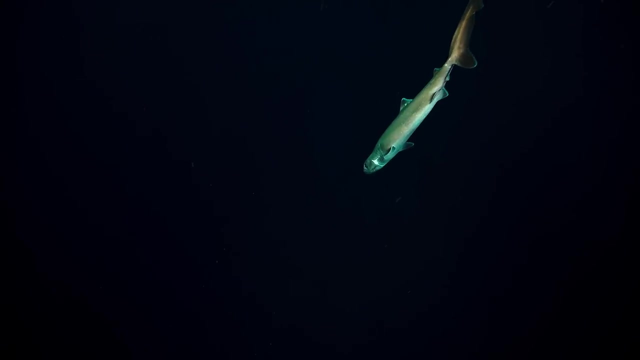 For nearly all creatures of the Twilight Zone, there is one thing that gives them away to predators: When they are seen from below, their dark silhouettes stand out against the low levels of downwelling light. But this challenge has given rise to some rather creative methods of camouflage. 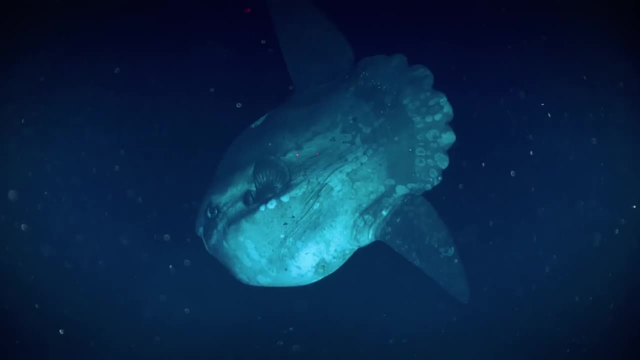 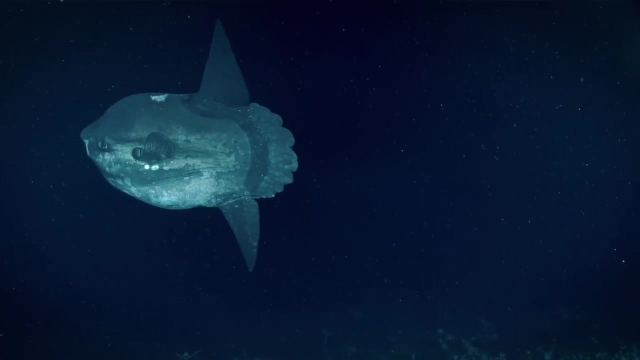 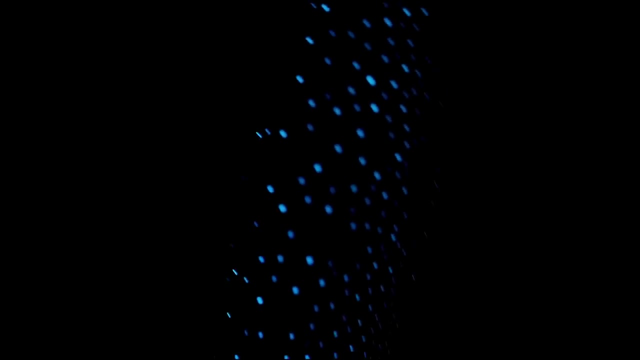 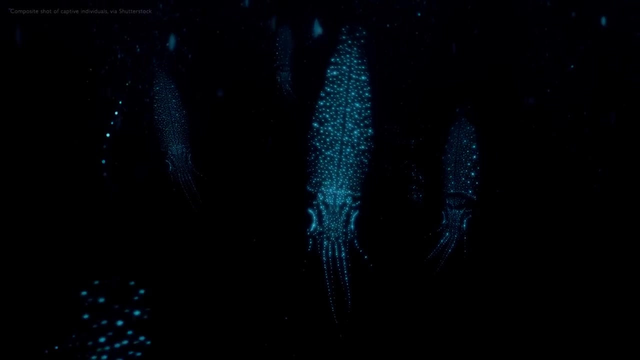 Some use countershading, expressing darker pigments on their upper body and lighter colours below in order to blend in from all angles. Others achieve this effect to a greater degree by emitting their own light, Bioluminescence, produced from glandular organs called photophores that line their bodies with a pattern of glowing dots, like those of the firefly squid. 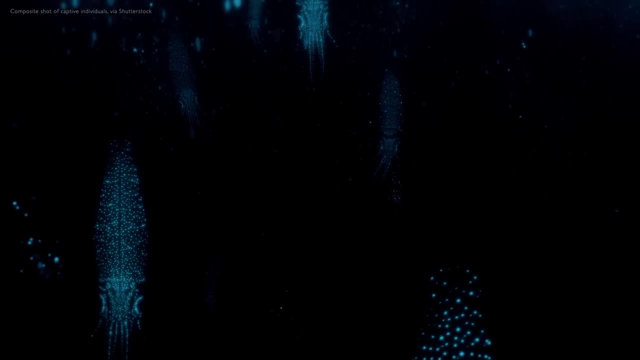 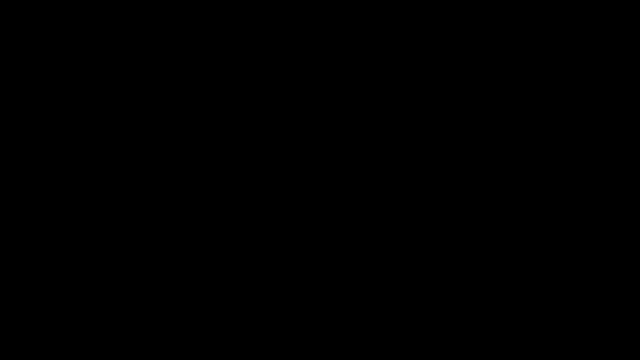 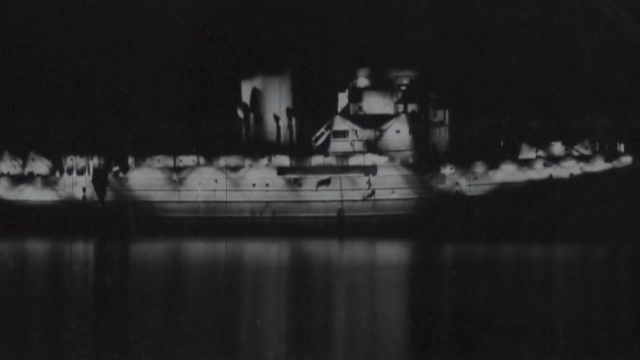 As they ascend, they increase the intensity of their lights to match the levels of sunlight radiating from above. This principle even gave rise to a naval tactic called Diffused Light Camouflage, where counter-illumination was used to make ships blend in against the backdrop of the night sky. 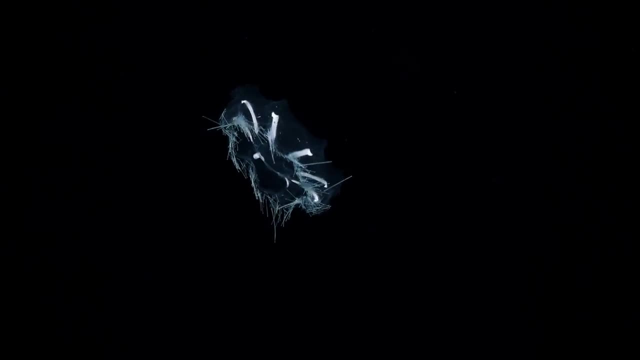 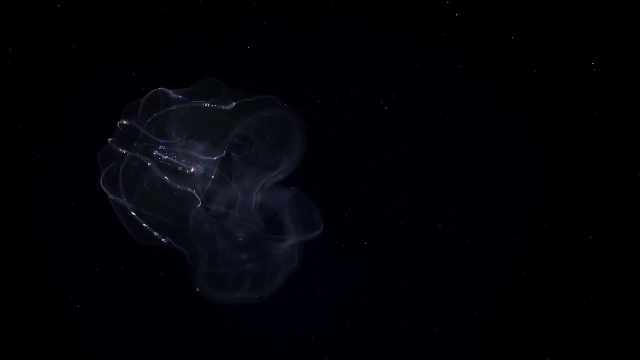 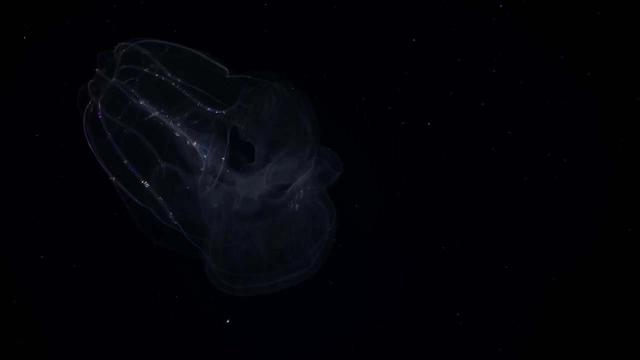 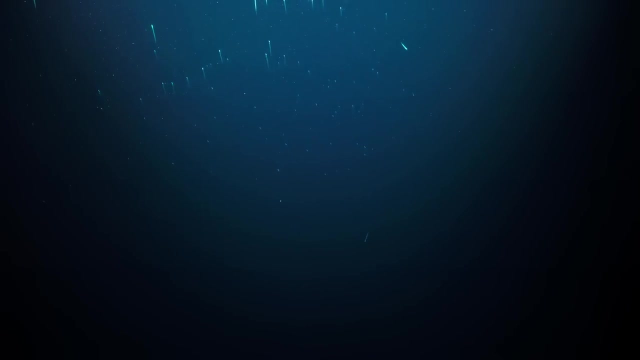 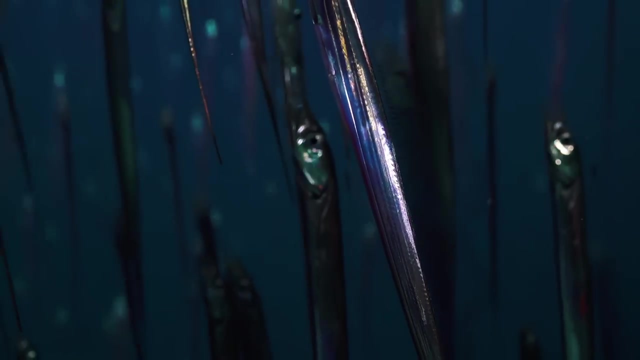 Counter-illumination is one of three dominant methods of camouflage that midwater species employ to resemble their environment. The second is transparency, like we saw in the planktonic drifters and glass squid. And the third is silvering, Lacking scales and instead covered with highly reflective skin consisting of microscopic guanine crystals. 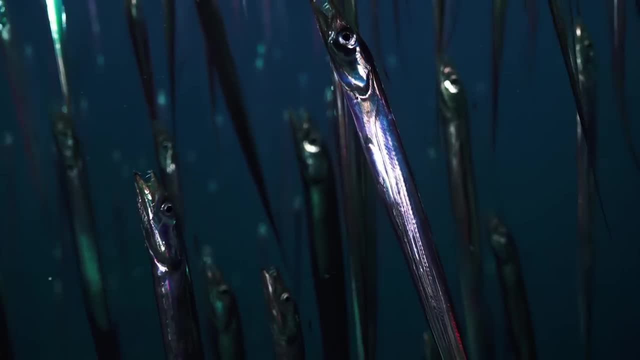 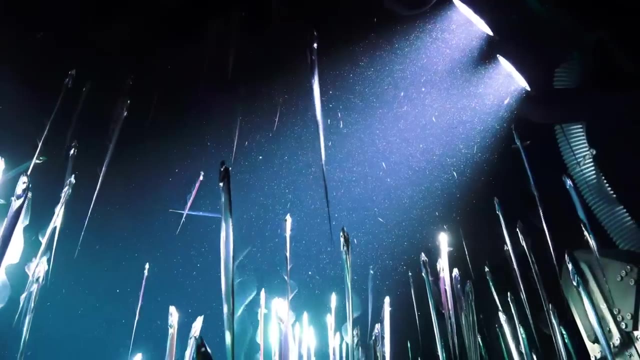 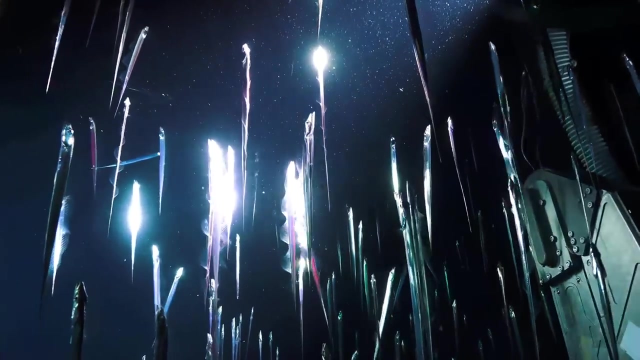 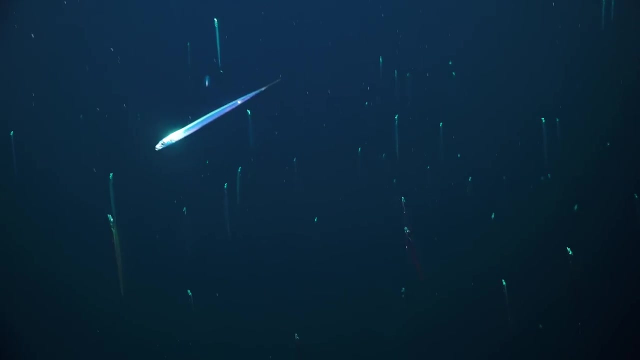 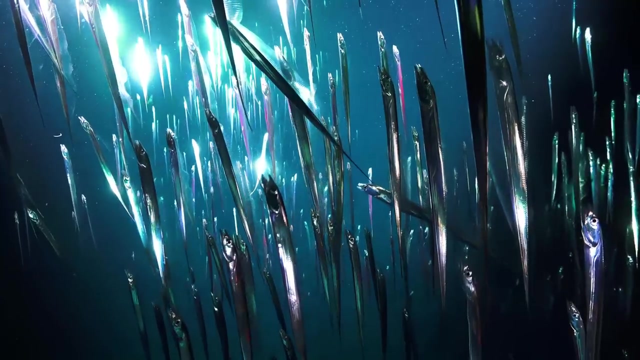 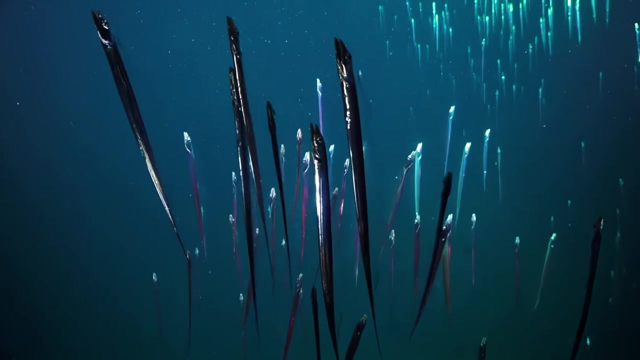 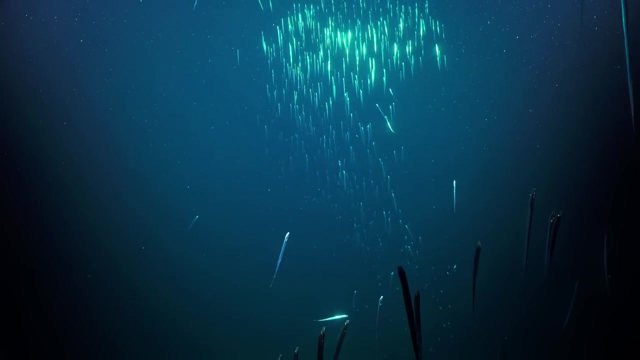 the needle-like cutlass fish resembles polished steel. This effectively imitates transparency, since, although it stands out in the lights of an ROV, the vertically oriented mirror makes these fish invisible from the side in the dusky water. It's so effective that almost all upper-ocean fish, including sardines and herring, use silvering to blend in. 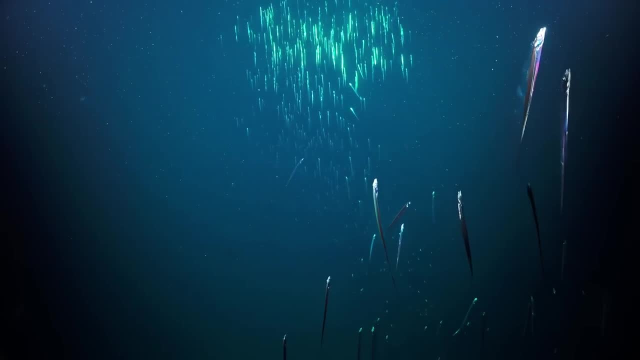 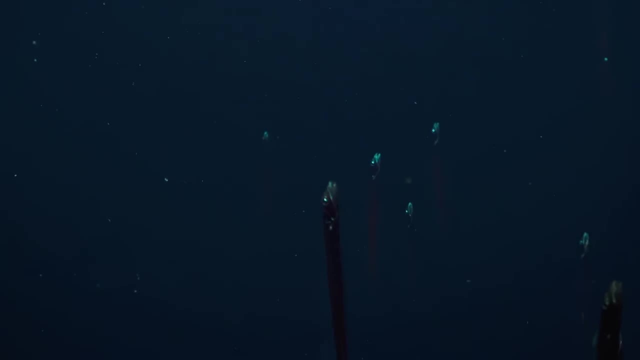 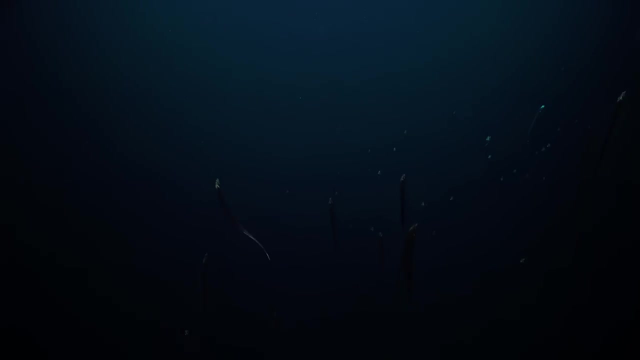 The second method is a method that allows the fish to blend in. The third method is a method that allows the fish to blend in. The fourth method is a method that allows the fish to blend in. The fifth method is a method that allows the fish to blend in. 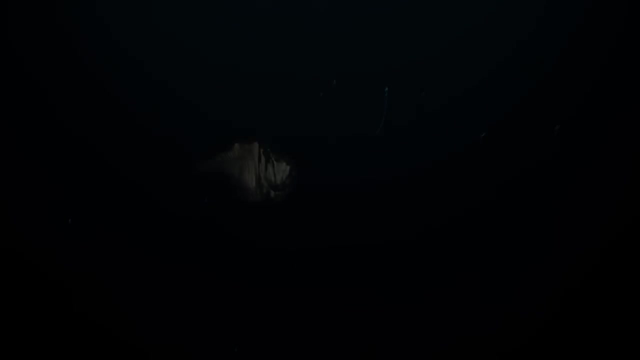 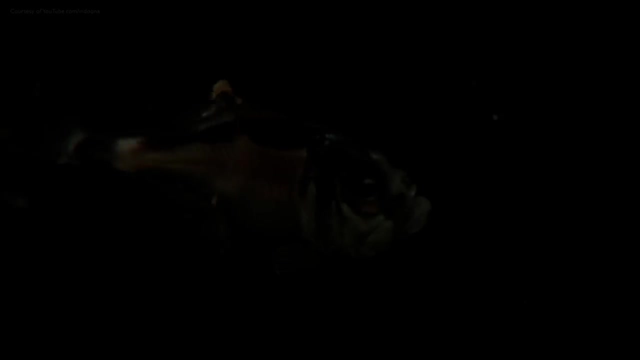 The sixth method is a method that allows the fish to blend in. The fifth method is a method that allows the fish to blend in. The hatchet fish has a laterally flattened body just a few millimetres thick, making it almost invisible from head-on and below. 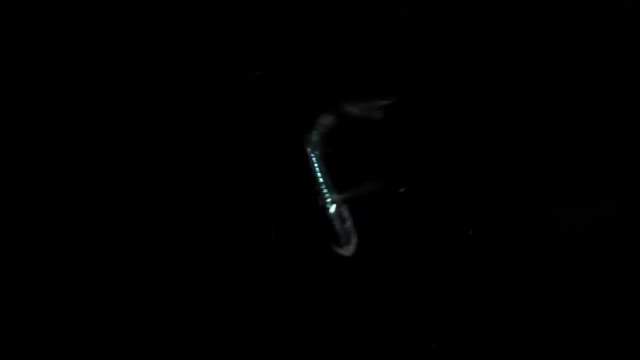 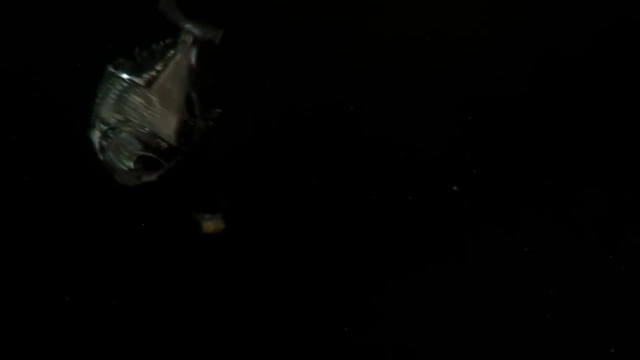 The fish is also able to move around in the water, and on its skin, the guanine crystals are perfectly spaced to scatter any light. And on its skin, the guanine crystals are perfectly spaced to scatter any light, But they also manipulate this light and funnel it downwards towards a set of photophores on its belly. 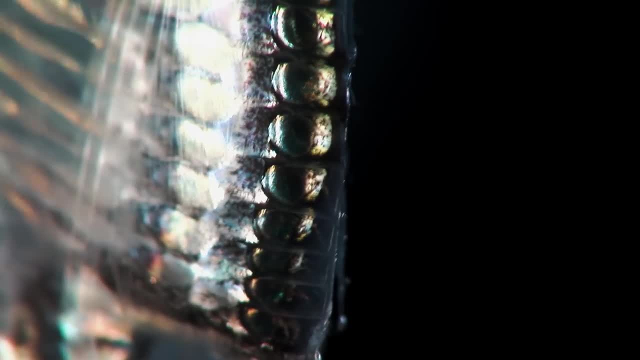 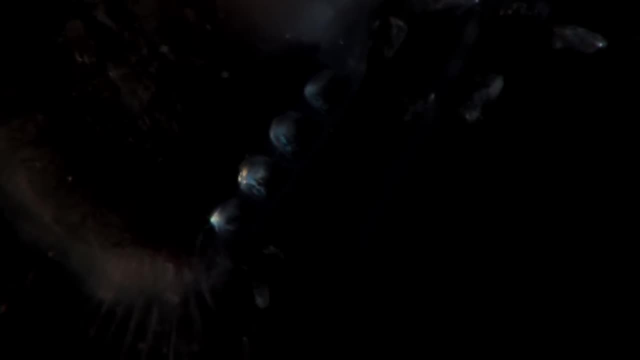 But they also manipulate this light and funnel it downwards towards a set of photophores on its belly, where it contributes to their counter-illumination. This serves a dual purpose for towards the deeper extent of their range. This serves a dual purpose for towards the deeper extent of their range. 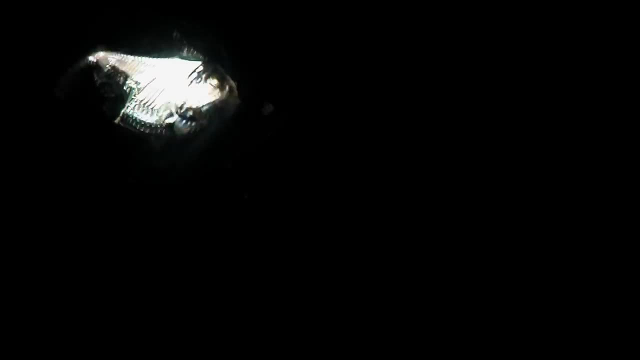 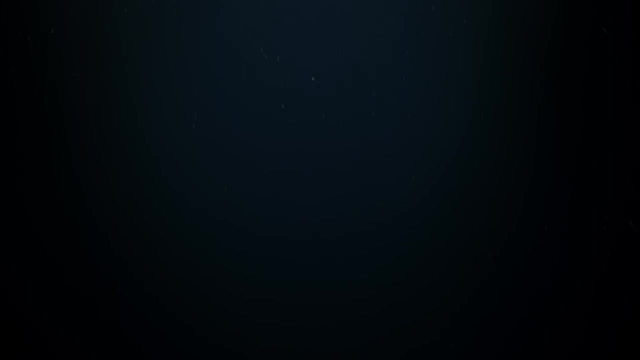 the downward scattering of light via their photophores may throw off the searchlights of midnight predators. the downward scattering of light via their photophores may throw off the searchlights of midnight predators. Silvering is found in cephalopods too. 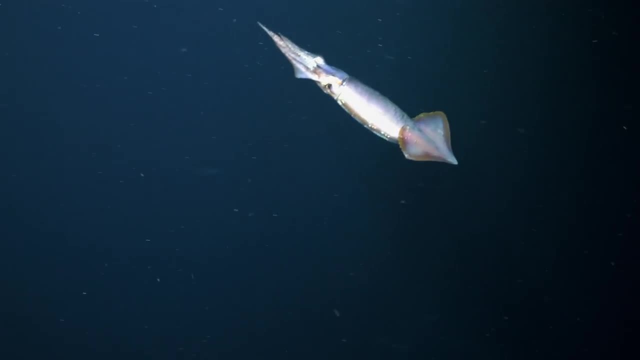 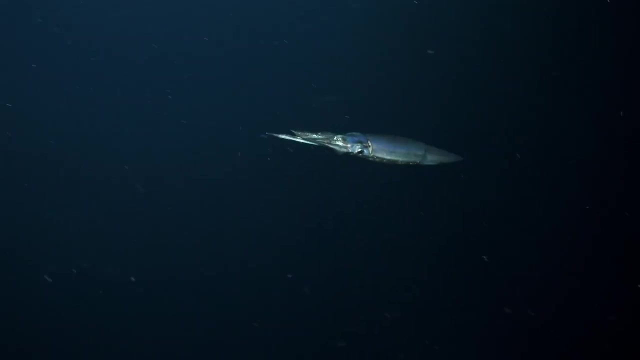 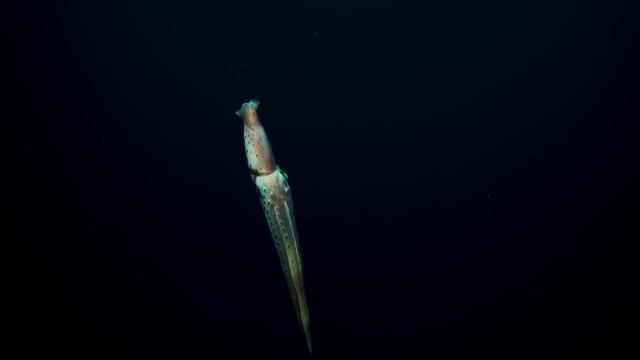 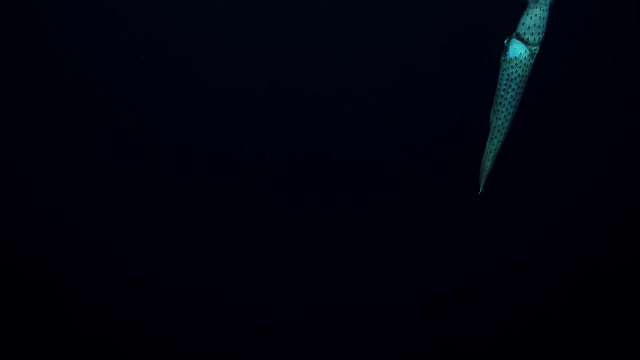 using not guanine but proteins called reflectins to create a mirror-like effect. One squid species has undergone the deep-sea equivalent of extreme body modifications. This is the cockeyed squid. One of its eyes is very big and the other rather small. 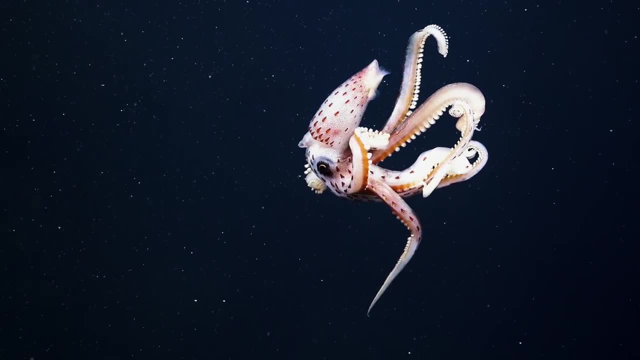 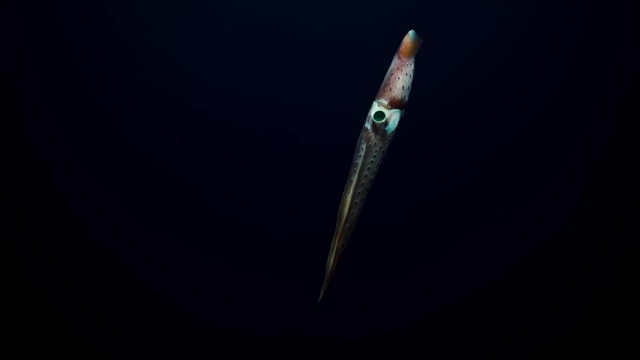 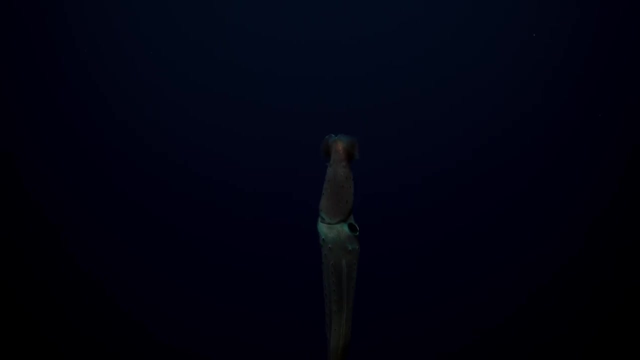 It positions itself in the water column so that the small eye looks downwards, spying for flashes of bioluminescence in the blackness below. Meanwhile, the large eye looks up. A bulbous tubular shape, takes in as much downwelling light as possible and a yellow 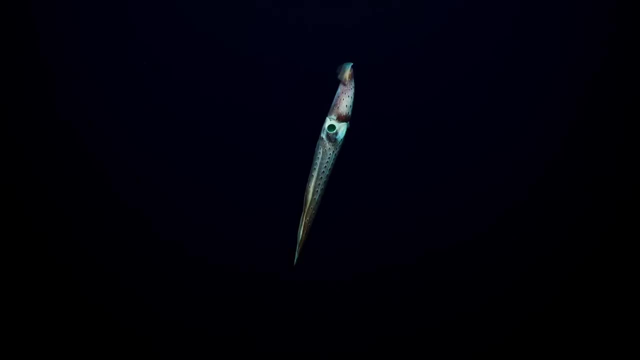 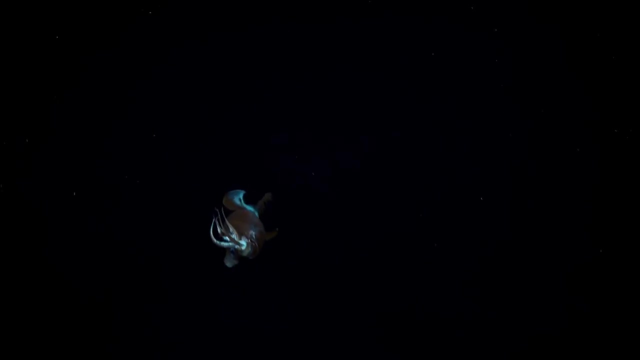 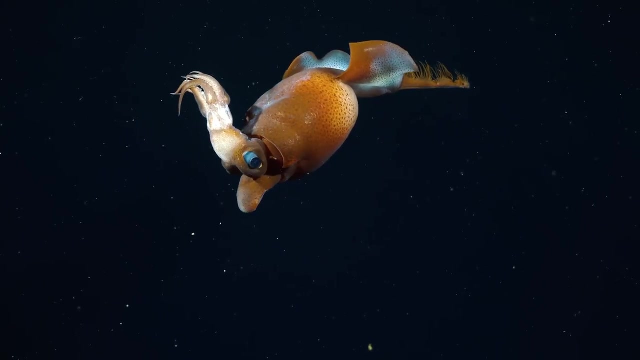 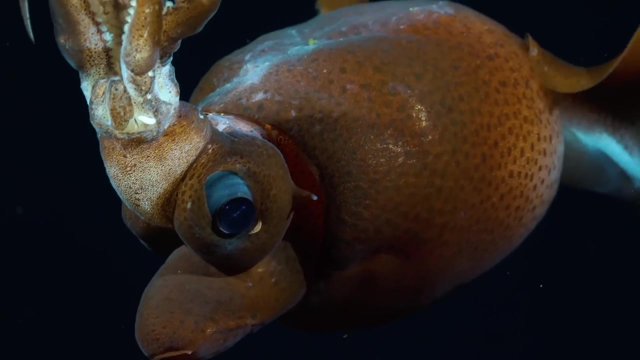 lens may allow it to see through the counter-illumination of prey. There's a reason why so many adaptations here converge on looking upwards and taking in more light. By living at an intermediate depth, creatures of the twilight zone have an advantage: The light levels are low enough that the gloom provides a level of protection, but just enough. 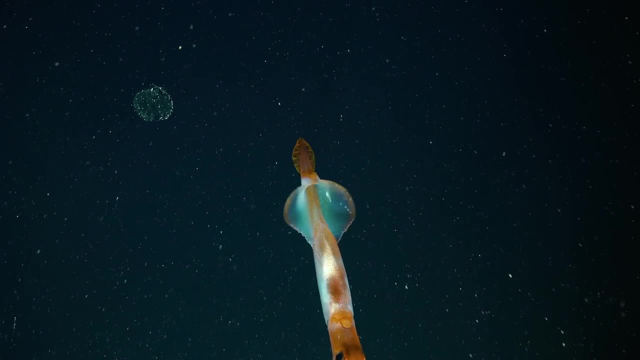 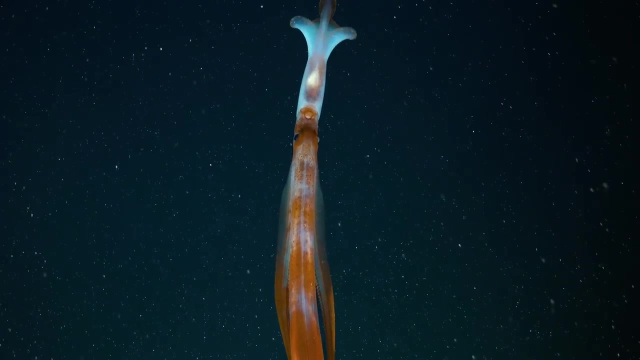 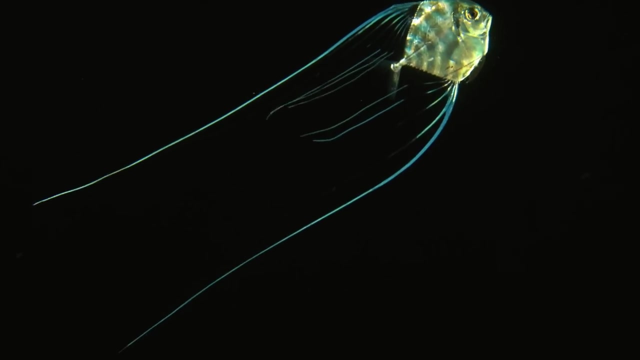 light remains that animals can use their remarkable light sensitivity to identify the coming of the night. A time when predators of the surface waters become less active and, in response, every night the denizens of the deep pay a visit. A time when predators of the surface waters become less active and, in response, every 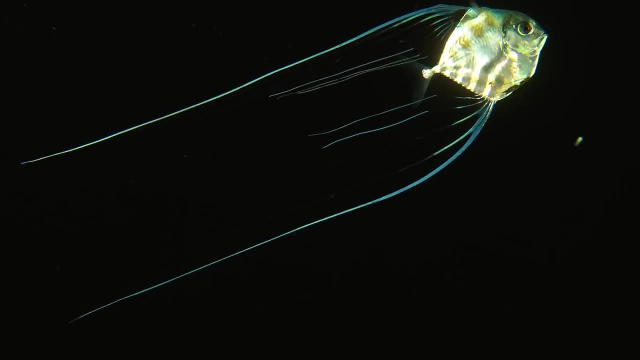 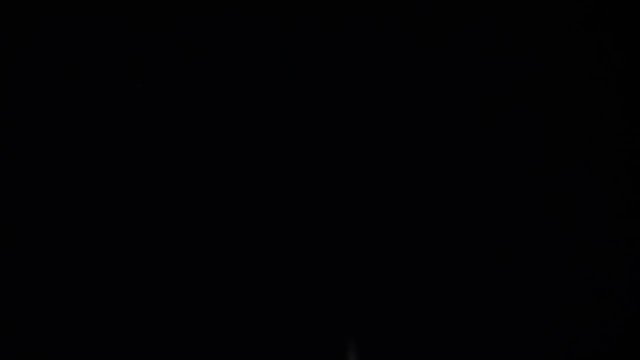 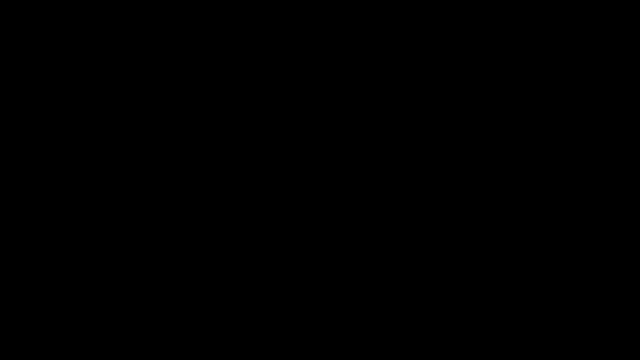 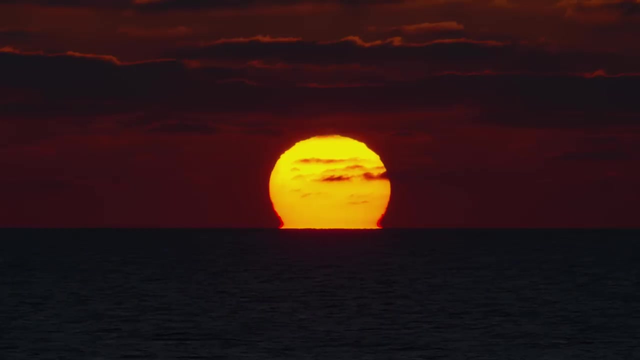 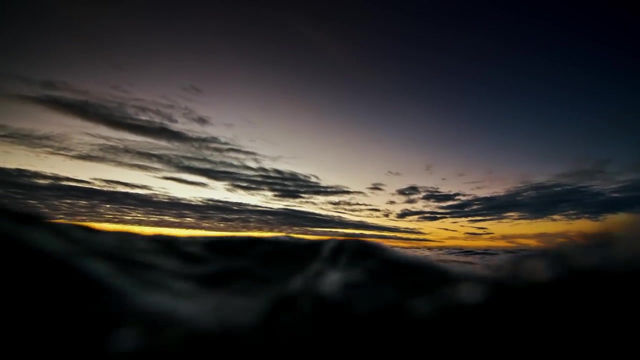 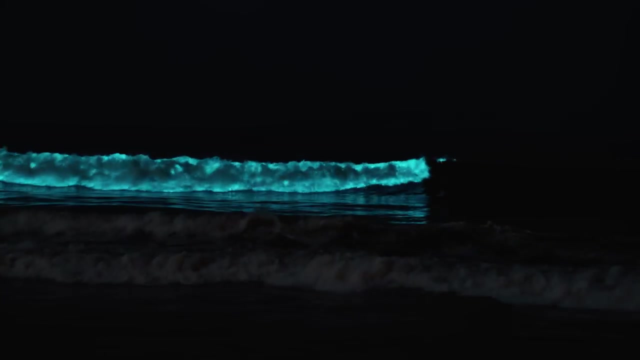 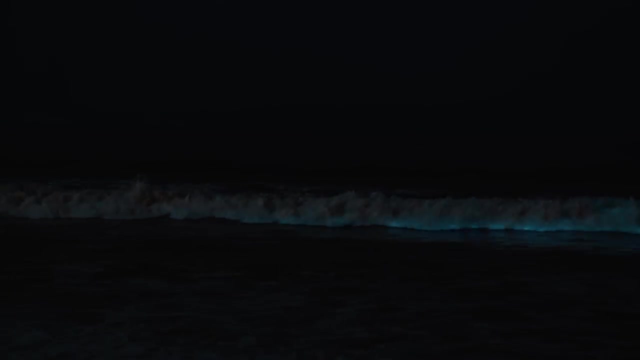 night, the denizens of the deep pay a visit to the shallows to feed on the abundant phytoplankton. It's a phenomenon called the Diehl Vertical Migration. The large-area structure was built in the 1850s and the water was one of the main sources of 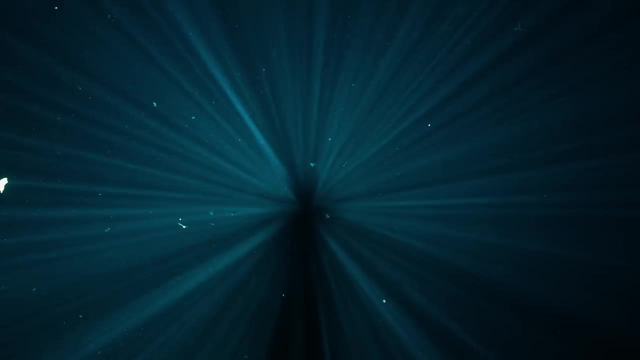 daffodils. There are millions of them and the very natural selection they find is increasing every day. The various species, and they are free from harm. The humans and the animals themselves are free from harm. They have no right to harm. 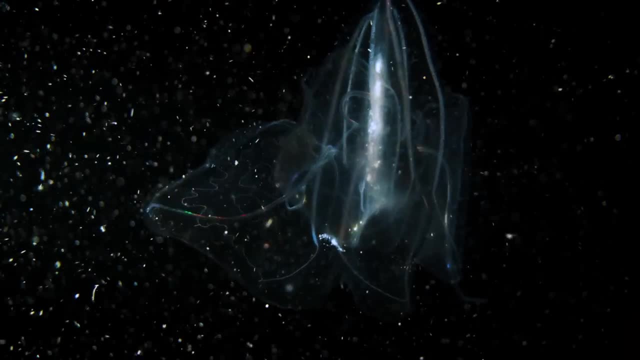 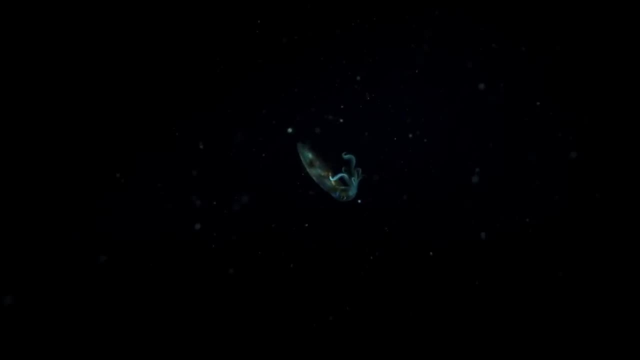 They have no right to harm. As night falls, vast numbers of animals rise from the depths of the Mesopelagic under a blanket of darkness. Deep sea jellyfish, siphonophores, squid and many others gather near the surface to feed. In their wake the entire food web of the Mesopelagic follows, and up from the depths come the innumerable sharks, fish, squid and all manner of deep sea predators. These vertical migrations unite planktonic organisms and their predators. 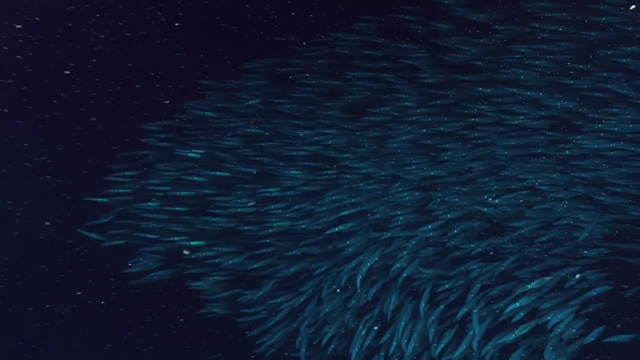 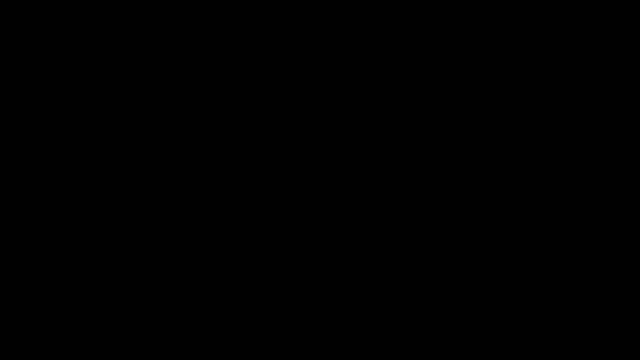 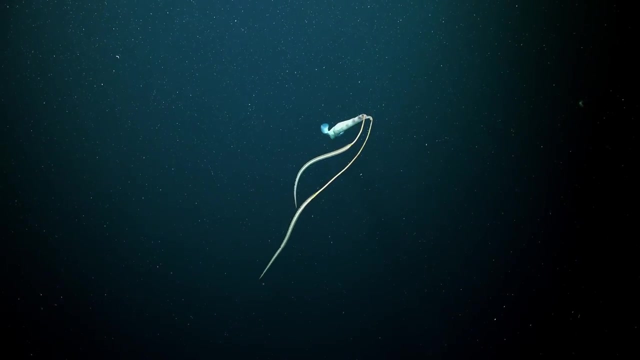 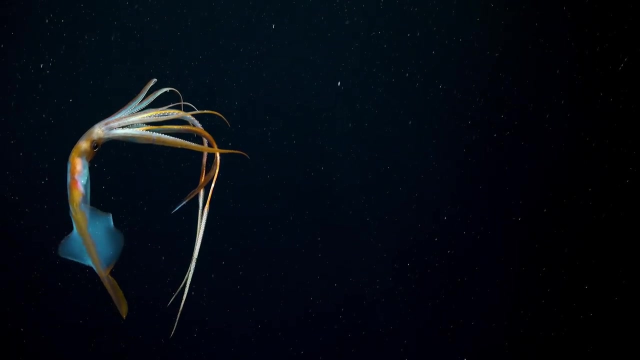 in a constant cycle of movement. Together, they form the largest synchronous migration on planet Earth. It's been postulated that animals may migrate at night to remain in their preferred light climate or isolume Using this ability an estimated 5 billion metric tonnes of organisms. 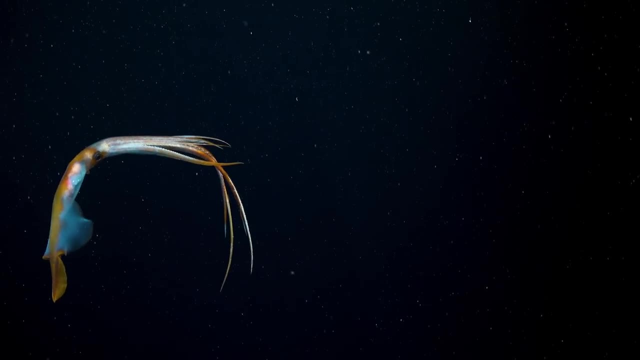 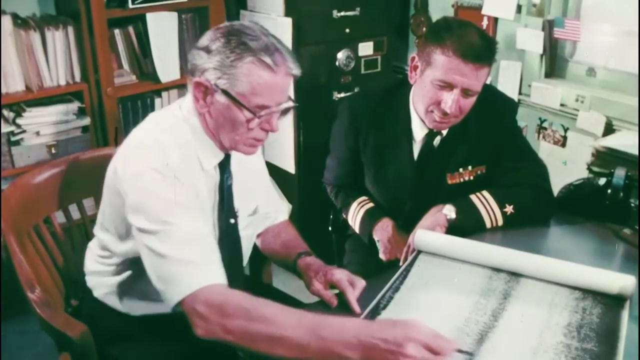 migrate up towards the surface every night and migrate back down come the dawn. A mass movement so large that it is impossible to predict how long it will take for them to migrate, and a mass movement so dense that it was first discovered when echo-sounders on board. 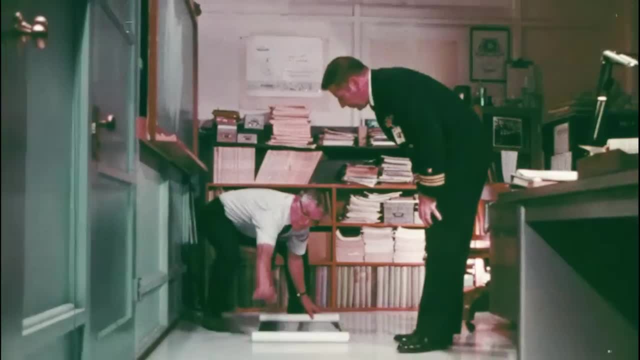 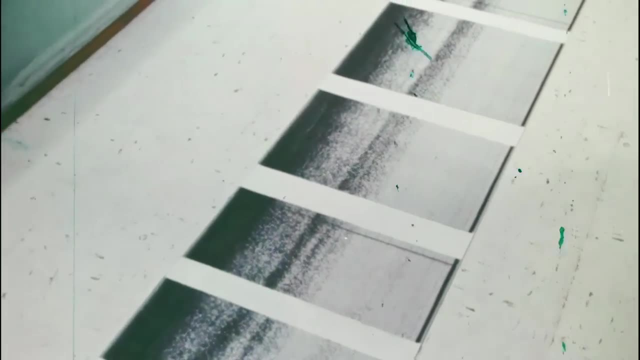 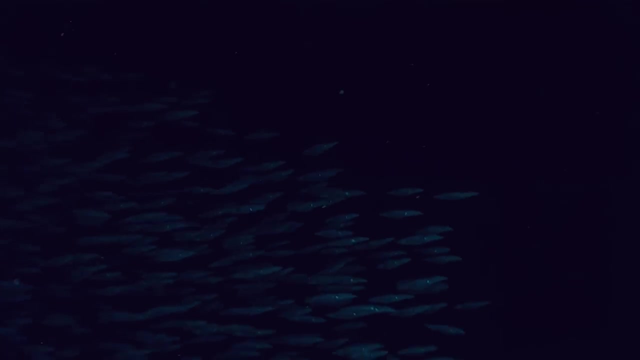 World War II, US Navy vessels detected the gathering of animals as a mysterious second floor in the ocean, far shallower than the ocean bottom was thought to be As a gathering of creatures from vastly different groups. the migration is a vertical feast that fuels the ocean's food web. 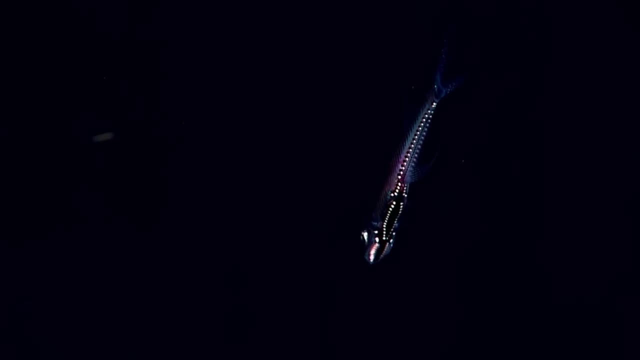 Take the lanternfish, for example. They are the most widely distributed and abundant vertebrates on the planet, with an estimated global biomass of up to 16 gigatons and accounting for 65% of all fish biomass in the deep ocean. 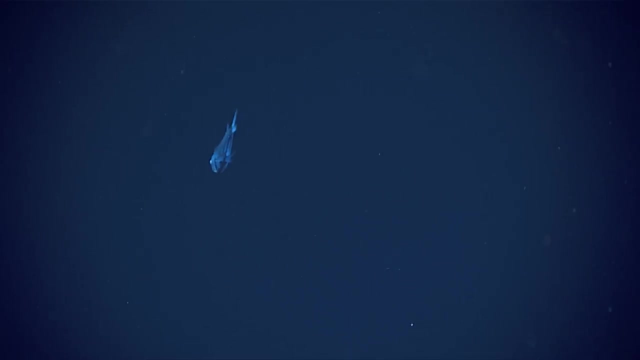 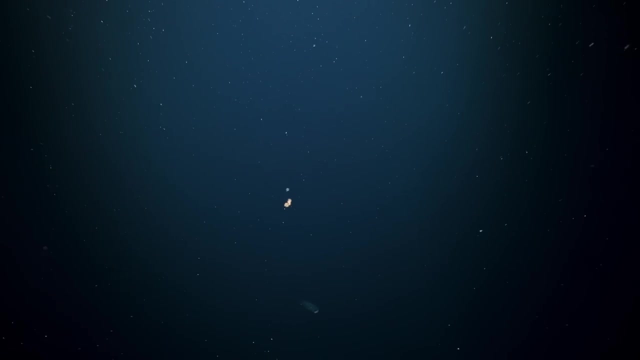 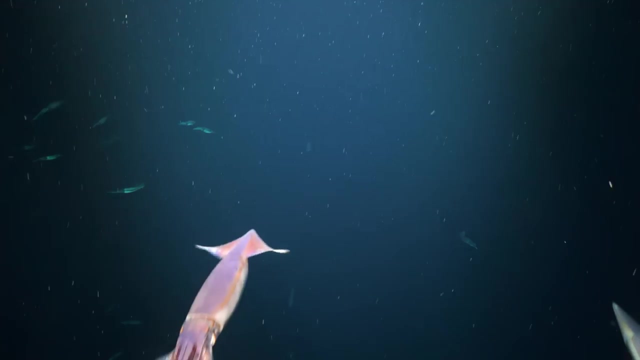 Because of this, they are a crucial food supply for many animals and a fundamental link in marine food webs. Their most notable predators are the red devil squid, which gather in shoals of up to 1,200 in individuals near the surface every night. 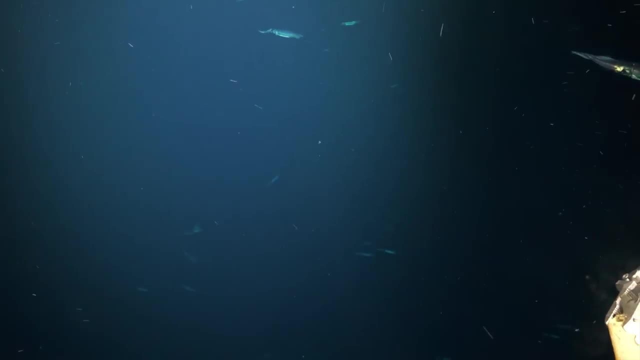 Their entire bodies flash red and white to signal to other members of the shoal. though the reason is unknown: It may be an invitation to reproduce, or perhaps it's to warn others not to get too close, For when the supply of lanternfish runs out, they turn on each other. 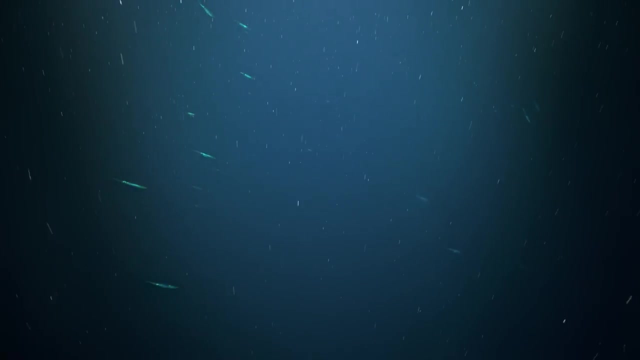 Cannibalism is rife among red devils, as studies of their stomach contents revealed the remains of fellow squid in a quarter of specimens. This could explain how they're able to grow so large so quickly, reaching well over a metre long in less than a year. 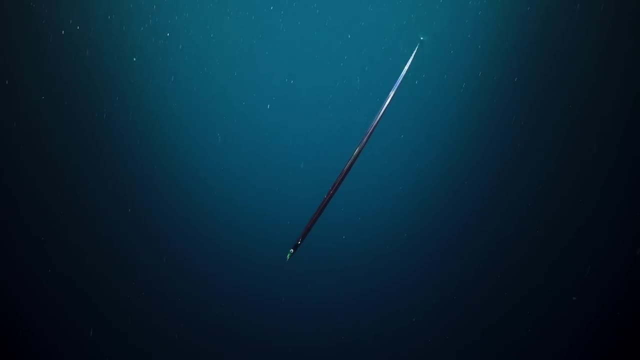 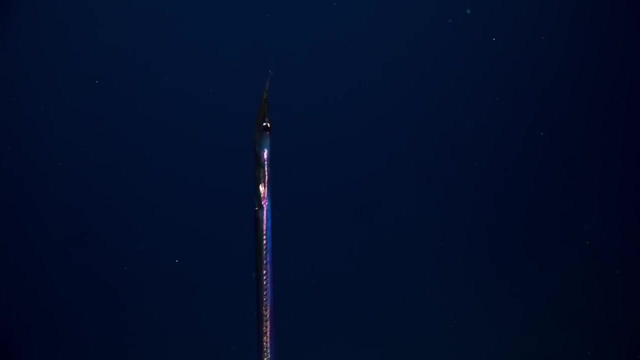 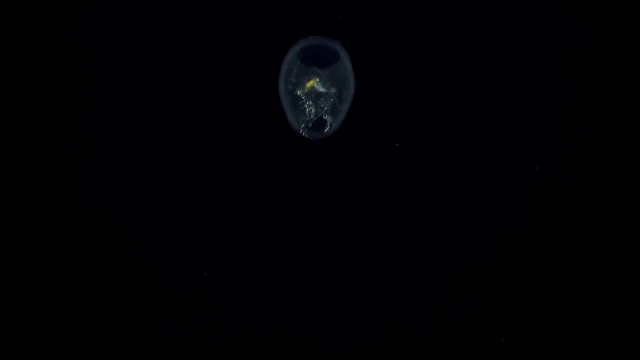 The 24-hour cycle of the vertical migration is one of the great forces that shapes the diversity and productivity of entire oceans. It shows off the ability of life to make use of cycles and queues that allow them to exploit resources in different habitats. Life in the deep sea would be nowhere near as diverse without the migration. 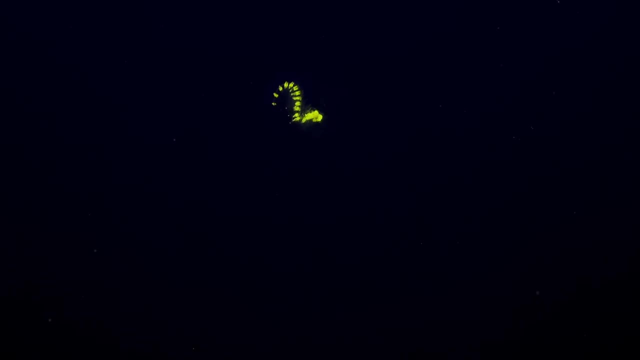 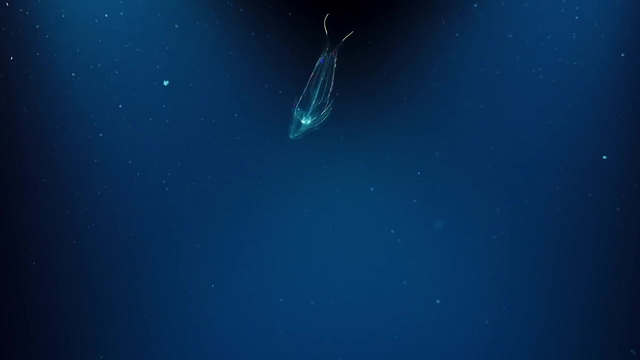 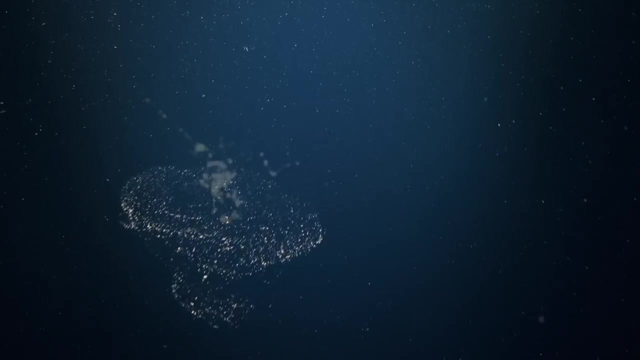 It fulfils an important role in the biological pump, since the phenomenon sees midwater organisms feeding at the surface and bringing the acquired biomass, along with an enormous amount of carbon, down to depth. Here, a few different processes see the carbon make its way to the seafloor. 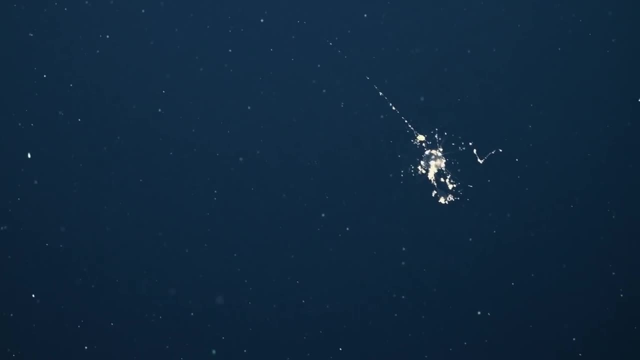 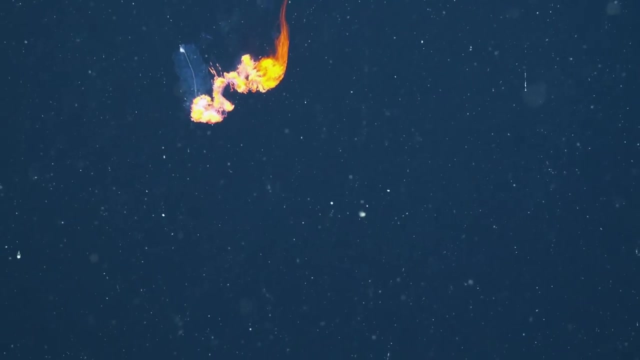 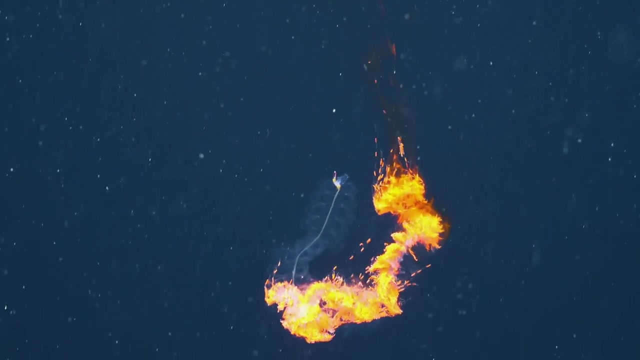 It enters deep food webs via predation and sinks through the water column in the form of marine snow and faecal pellets. This provides not only a means of sequestering carbon away from the atmosphere, but also a vital ecosystem service to deeper dwelling communities. 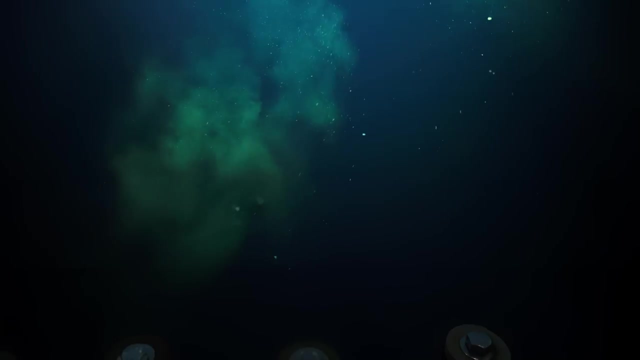 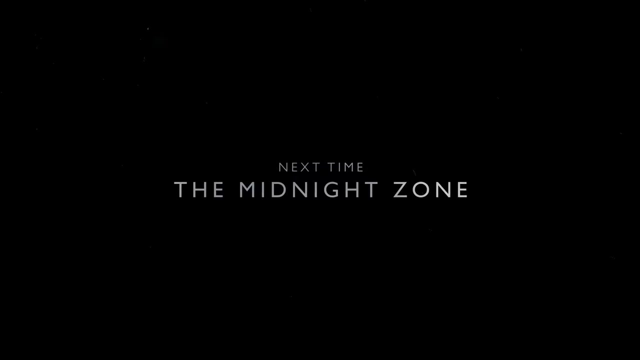 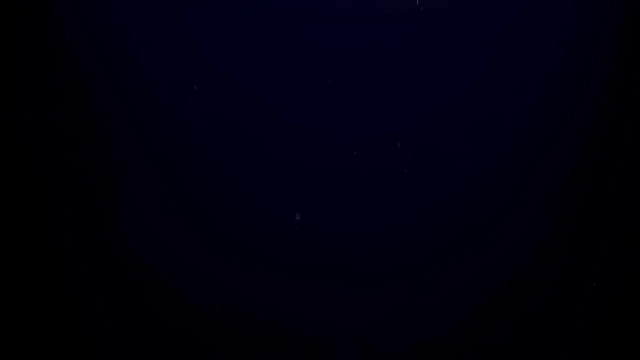 by providing a more direct pathway for food to reach the midnight zone below, where the total absence of sunlight makes vertical migrations far more challenging, And so, below around a thousand metres, there is a sharp decline in biodiversity. You could travel through this zone for hours and see very little. 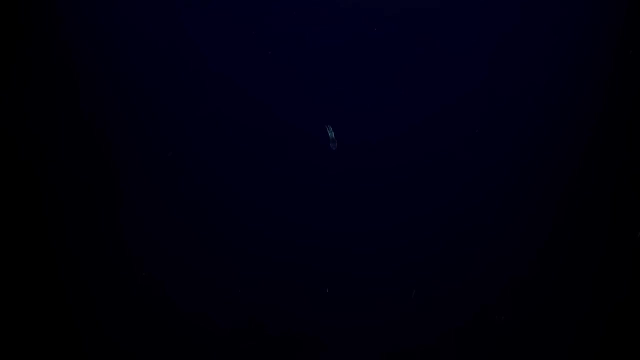 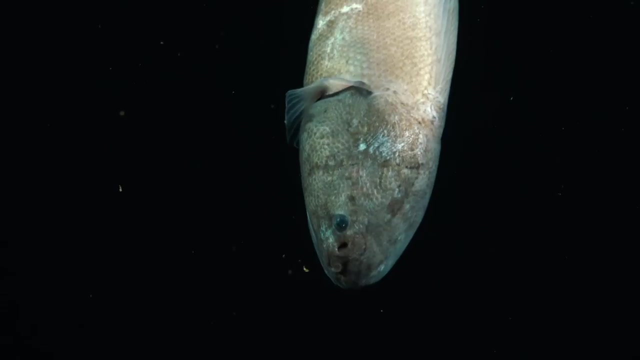 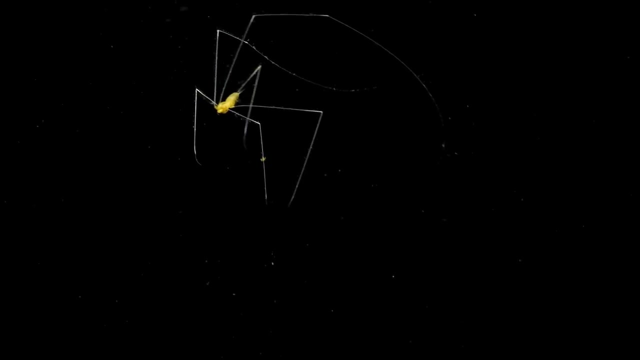 And yet it is not a dead zone, Far from it. Although a challenging world, it is also a stable one where the direct influences of the sun, the waves and the tides are not felt, Creating a habitat that has barely changed at all in millions of years.